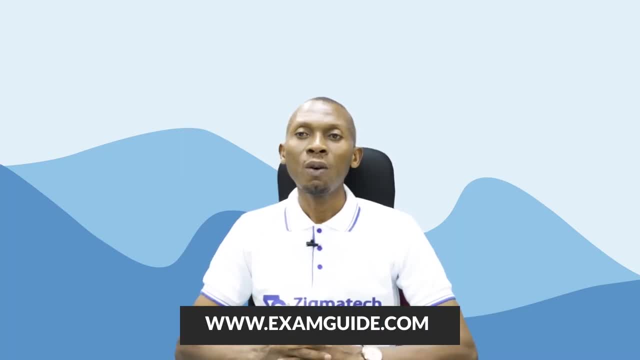 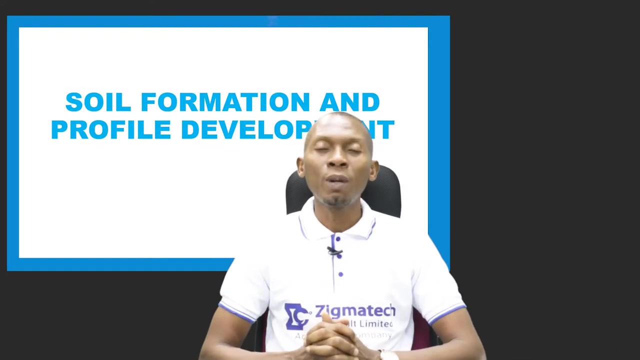 from wwwexamguidecom or Google Play Store. Please subscribe to our channel, Thank you, And turn on the notification bell to be updated on new videos Ready for today's class? Okay, let's get started. So this is the upper part of the earth on which plants grow. Now soil takes millions. 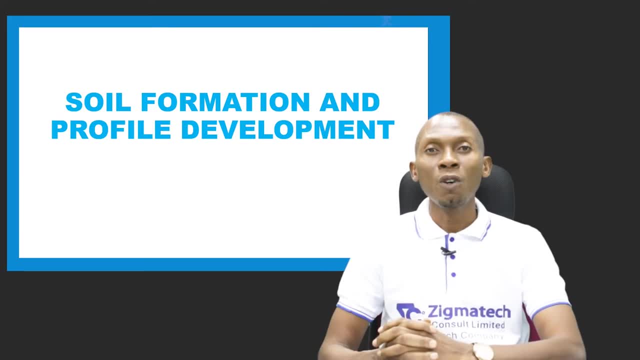 of years for it to be formed, And the soil can be formed as a result of the weathering of rocks, which has to do with the breaking down of rocks. Now, this can be achieved by fertilizing, mechanically or physically. It can also be achieved chemically, and it 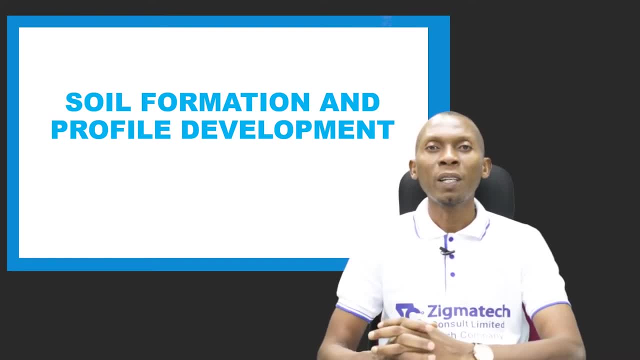 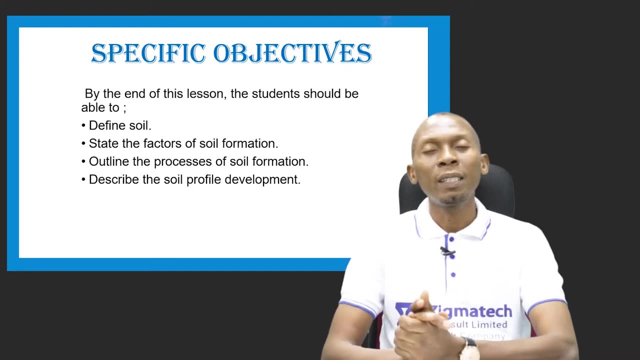 can also be achieved biologically. So in this topic we will be talking about soil formation and profile development. So our topic for today is soil formation and profile development, And by the end of this lesson we should be able to define soil. we should also be able to state the factors. 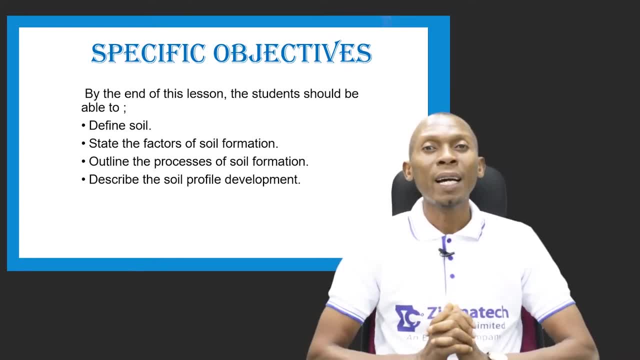 of soil formation. You should also be able to outline the soil. We should also be able outline the processes of soil formation And, finally, you should be able to describe the soil profile development. Now, what is soil? Let's take a look at the. 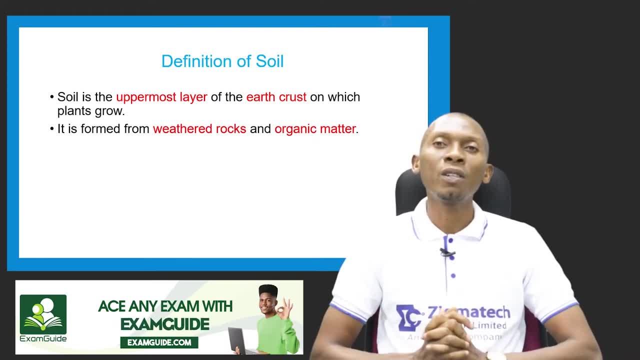 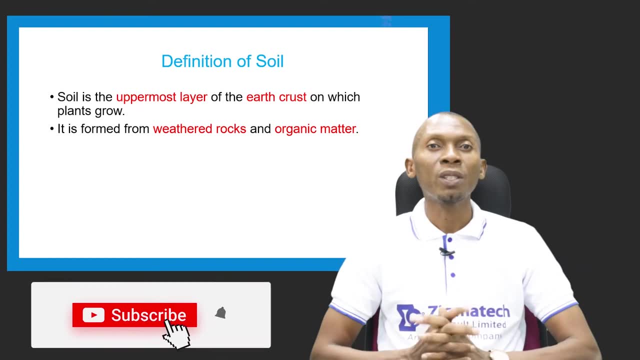 definition of soil. It said it's the uppermost layer of the earth crust on which plants grow. So the part of the earth where plants grow, which is the uppermost layer of the earth crust, is called soil, And soil is formed from the 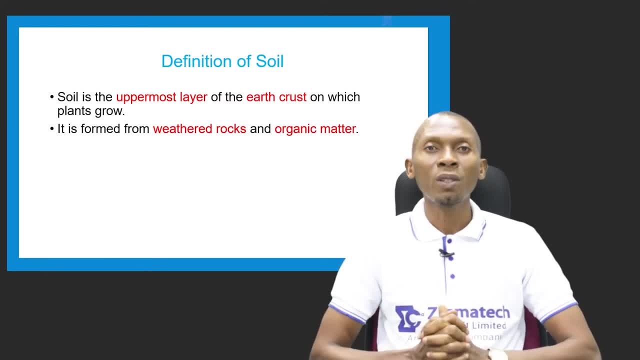 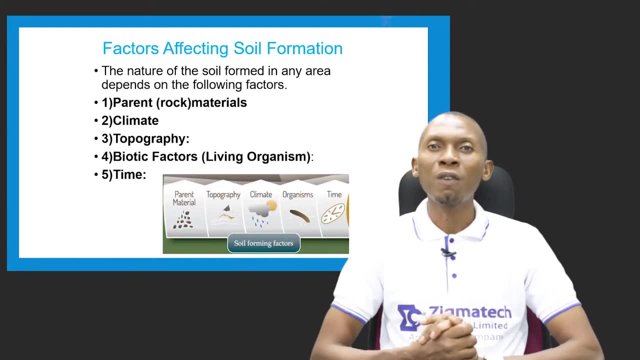 wetting of rocks, which has to do with the breaking down of rocks. So soil is formed from weathered rocks and organic matter. Now, what are the factors that affect soil formation? Now, the nature of soil that is formed in any area depends. 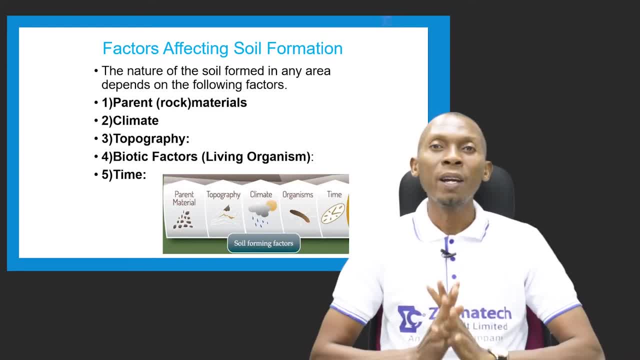 on some factors, and these factors include the parent material, which is the parent rock- Remember we said soil is formed from rocks- Also the climate, topography, biotic factors, which has to do with living organisms, and time. So these are. 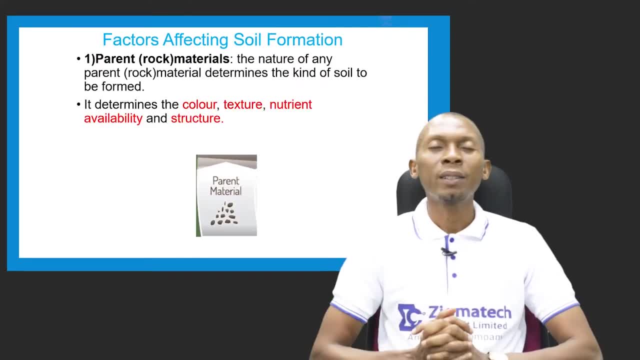 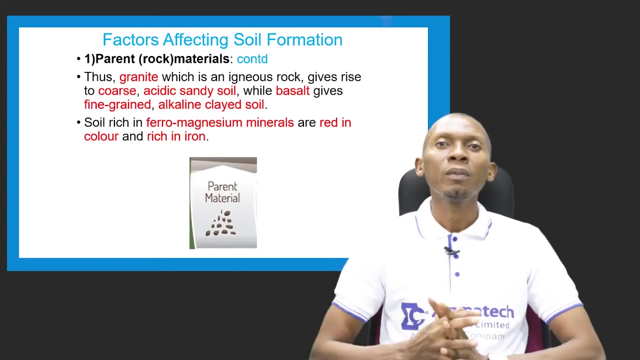 the factors that affect soil formation. Now, starting with the parent material, parent rock. Now, the nature of the parent material determines the kind of soil that is formed. So it's the parent material helps to determine the color, the texture, the nutrients available and the structure of the soil that is formed. 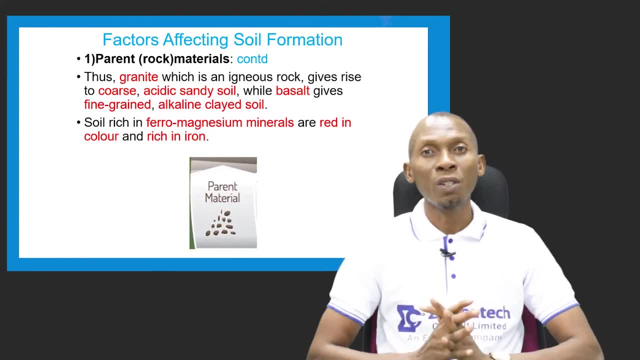 For example, we have granite, which is an igneous rock. This type of rock gives rise to a coarse and acidic sandy soil, while basalt, which is also an igneous rock, gives rise to fine-grained, alkaline clay soil. 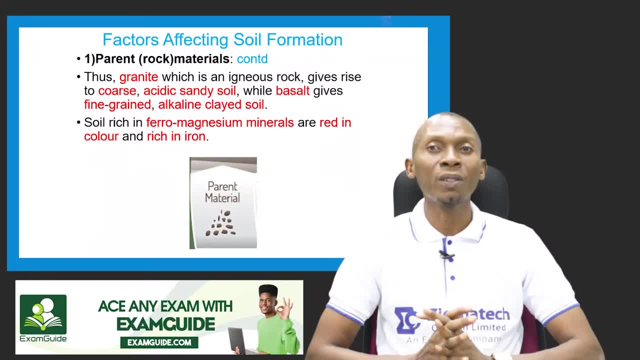 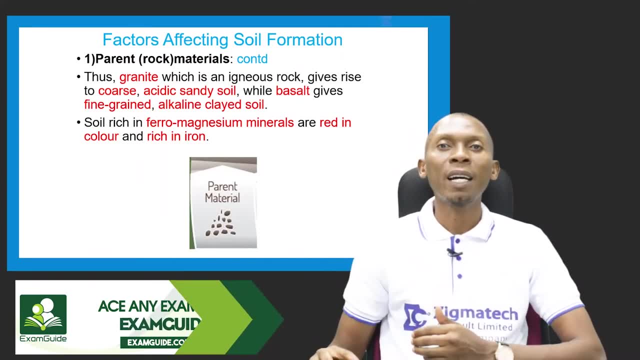 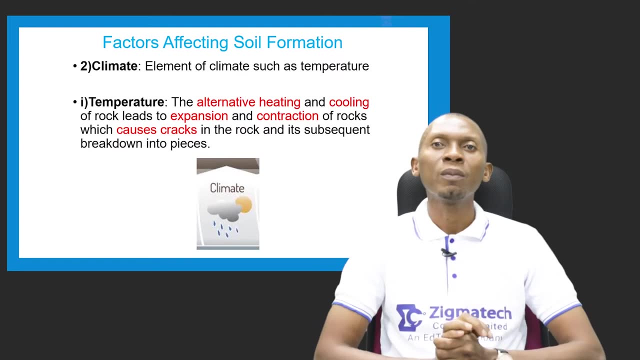 And soils that are also rich in ferromagnesium minerals are usually red in color and rich in iron. So we can see how the parent materials do affect the type of soil that is formed. We have climate as another factor affecting soil formation. Now, climate includes things like temperature. 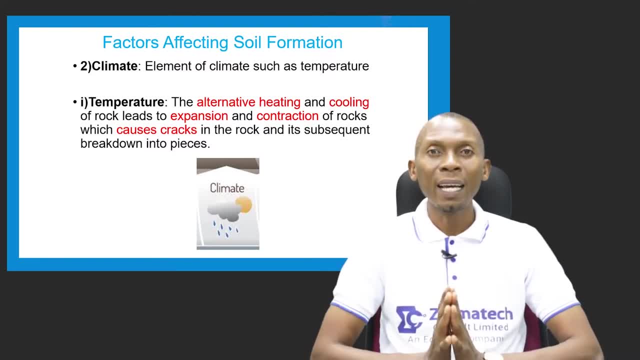 So when we look at temperature as a factor for that climate, how it affects soil formation, Now, temperature has to do with the alternative heating and cooling of rocks And as a result of this alternative heating and cooling of the rocks, we can see that 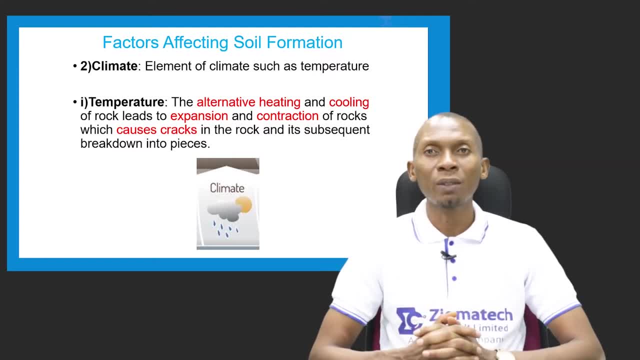 the rocks begin to expand and contract. So when it heats, it expands. When it cools, it contracts. So this heating and cooling alternatively causes the rocks to eventually crack. And once they crack, they break down into pieces, which now forms soil. 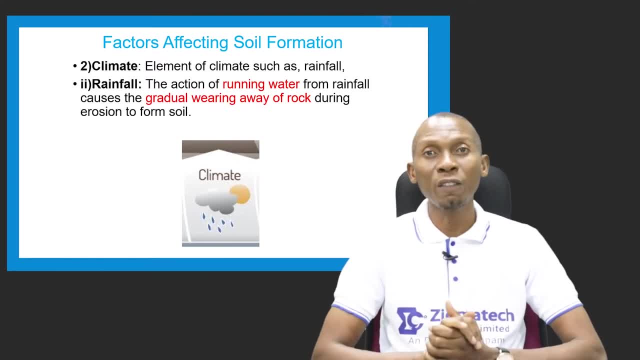 We also have another climatic factor, which is rainfall, And then rainfall has to do with the action of running water from rain, And as rain is a factor, it causes the rocks to crack. So we have a lot of different factors. The water is running. 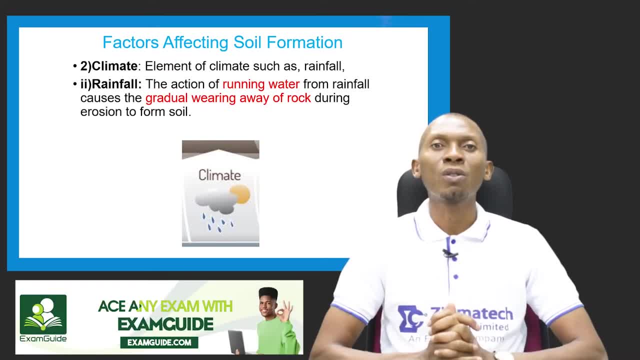 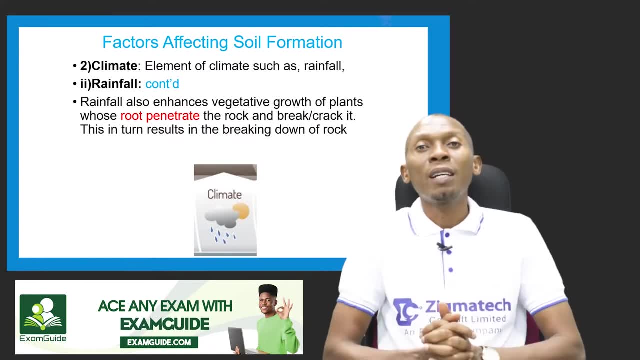 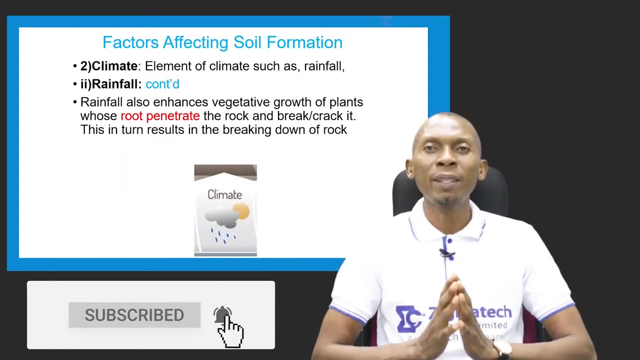 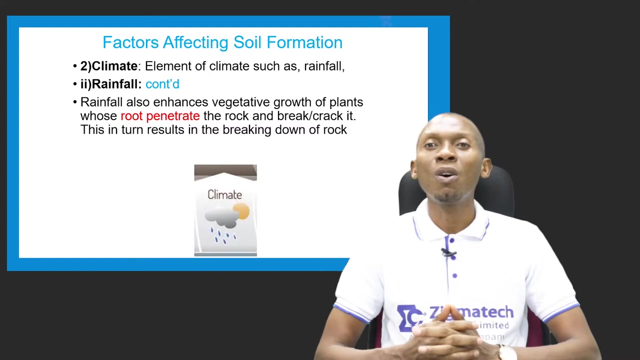 It causes some gradual wearing of the rocks during aeration, and this helps to form soil. Now, rainfall can also enhance vegetative growth of our plants, And as these plants grow, the roots of these plants are able to penetrate rocks. And once they penetrate the rocks, it can lead to the rocks becoming cracked or causing 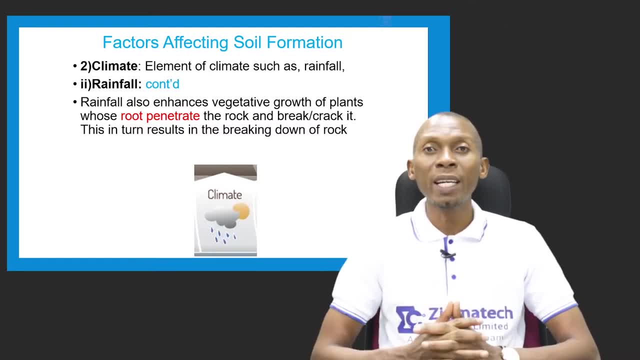 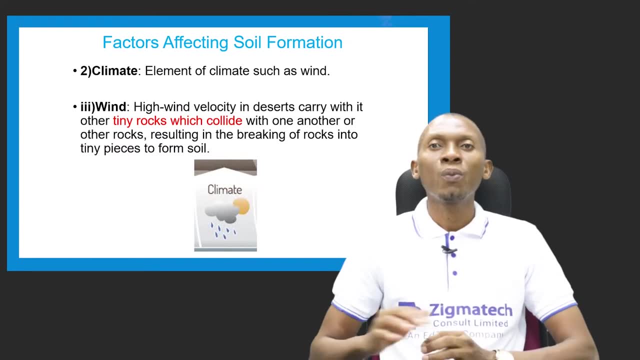 the rock to break or crack And, as a result of that breakage, the rocks will eventually break down to form soil. We have wind as another climate. So we've looked at temperature, We've looked at rainfall, Now we're looking at wind as a factor on that climate affecting soil formation. 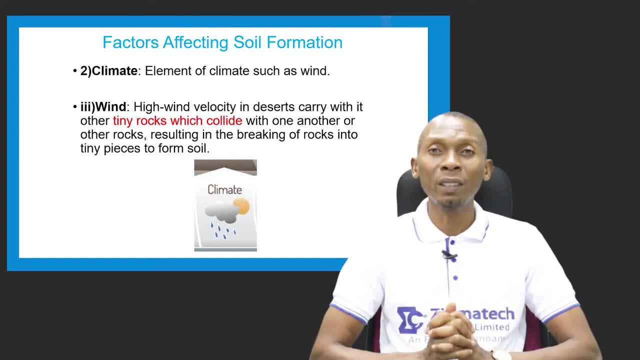 Now, wind has to do with high, As high wind velocity in desert areas can cause these tiny rocks, you know, to collide with one another. And as they collide with one another or other rock, it now eventually leads to the breaking of these rocks into tiny pieces to form soil. 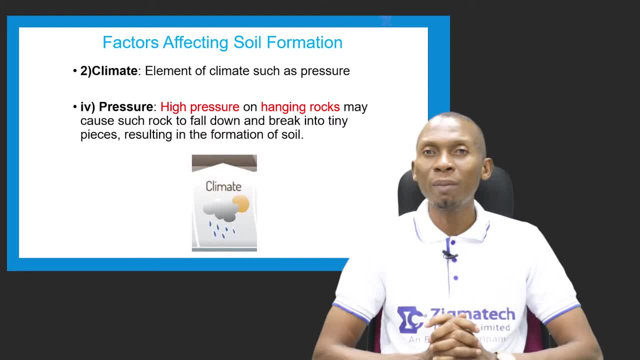 We have pressure as another element of climate that can affect or cause soil formation. High pressure on hanging rocks can cause these rocks to fall down, and when these rocks fall down, they can break into tiny pieces And as they collide with one another or other rock, it now eventually leads to the breaking. 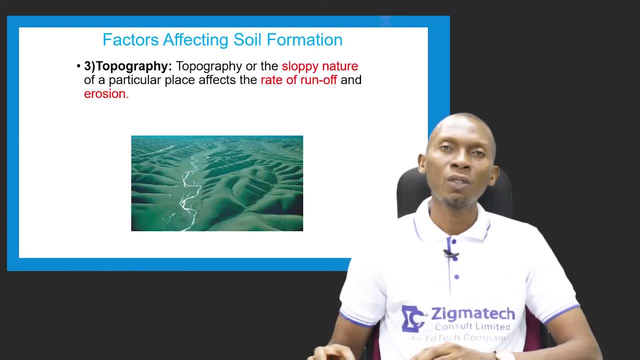 of these rocks into tiny pieces to form soil. We also have topography as another factor affecting soil formation. Now, topography has to do with the shape of the land. Now, if it's a slopey, it will encourage the runoff of water and this will now cause erosion. 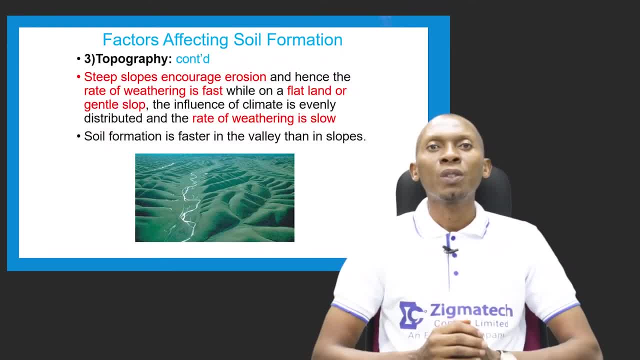 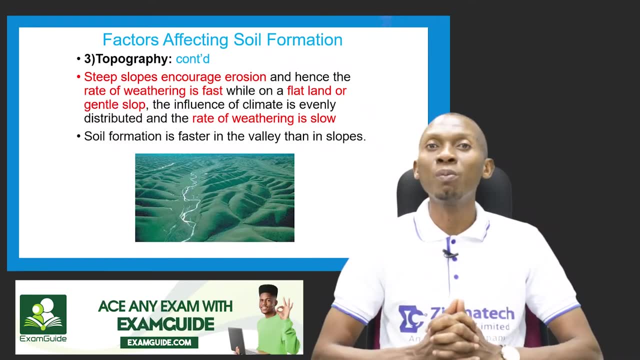 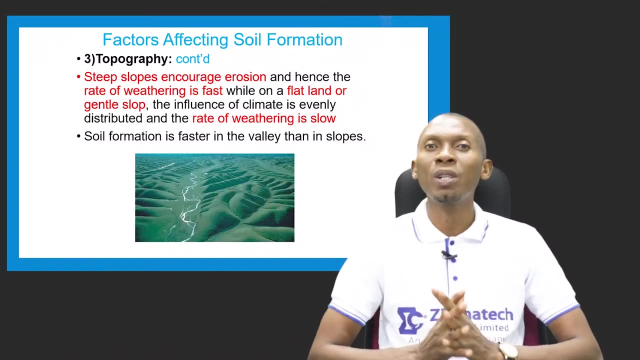 leading to the formation of soil. So we have. If the slope is steep, it will encourage erosion and once this happens the rate of weathering will be fast and weathering has to do with the breaking of rocks. But if the slope is flat- maybe probably a flat land or a gentle slope you will find. 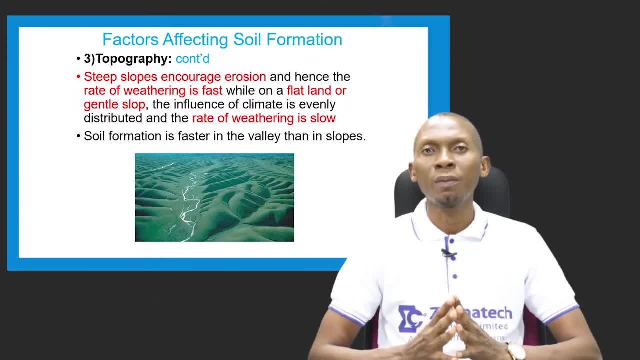 out that the rate of weathering will be slow because the climate will be evenly distributed and in this case the rate of weathering will be slow, as against if it is a steep slope. So soil formation is usually faster in valleys than in slopey areas. 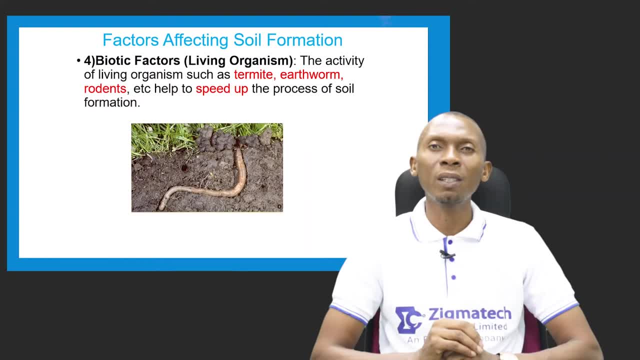 Biotic factors. Biotic factor: this has to do with the living organisms, and this has to This can also affect soil formation. Now, these living organisms here include organisms like termites, earthworms and rodents, and they also help to speed up the process of soil formation. 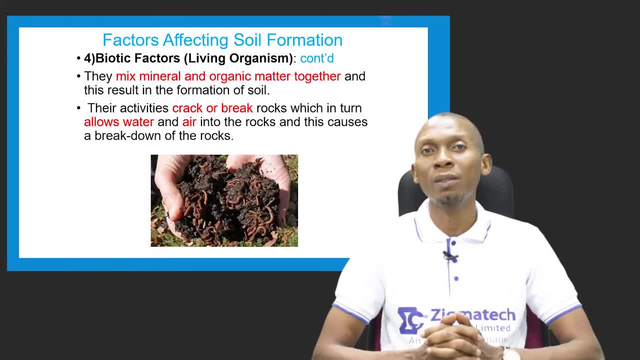 How do they achieve this? They help to mix minerals and organic matter together that are found and this results in the formation of soil And also Their activities. their burrowing activities can help also cause the rocks to crack and break and as a result of this, it allows those cracks and breakages or crevices causes. 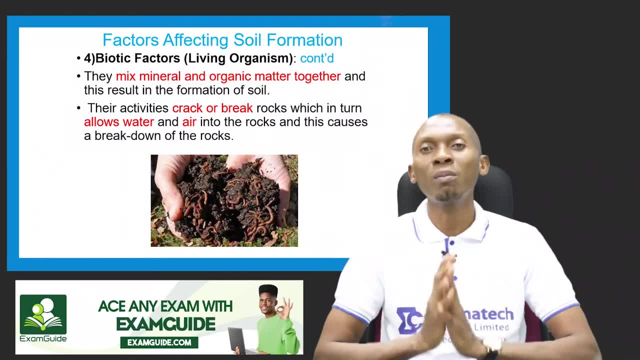 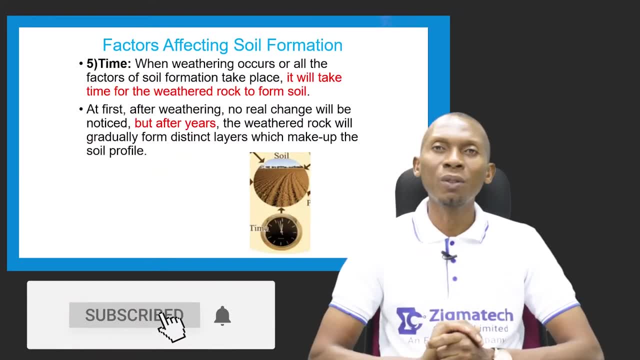 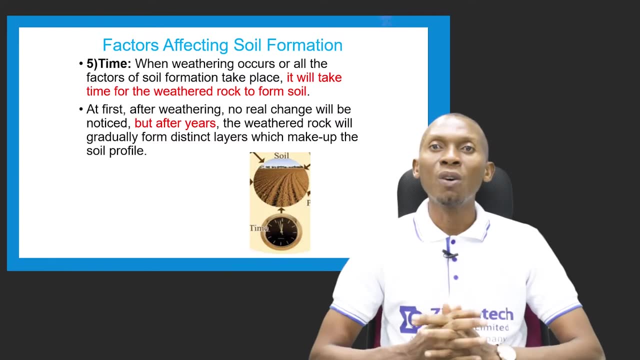 or allows water and air into the rocks, which will eventually break down these rocks to form soil. Time also is a factor that can affect soil formation, so it takes millions of years for soil to be formed. So when we're doing, When all this occurs, all other factors of soil formation take place. it will take time. 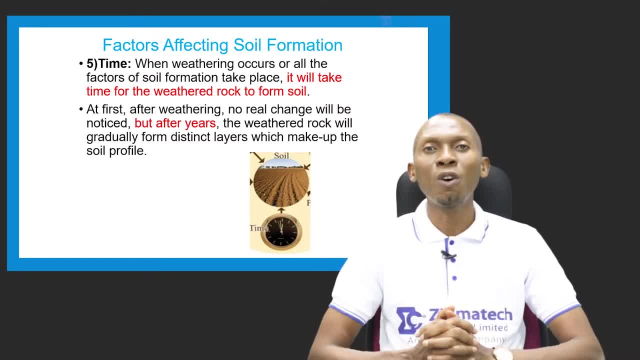 or it takes time for the weathered rocks to form soil. So eventually, when weathering takes place, you find out that there's really no change that is noticeable. but after a long time, after so many years, you find out that these rocks will gradually form distinct layers which now make up what is called the soil. 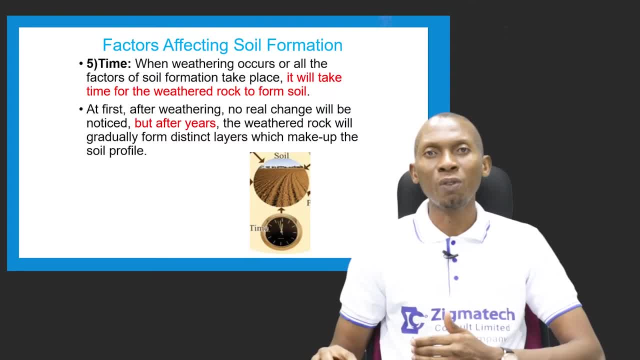 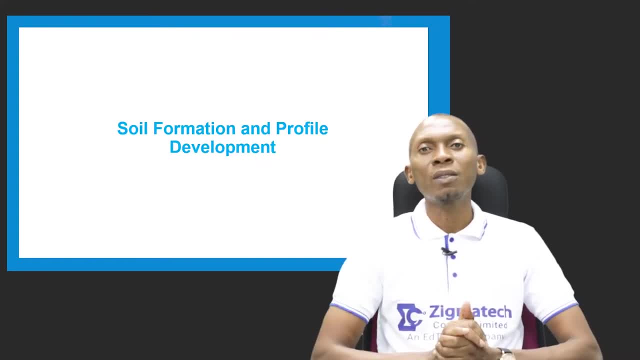 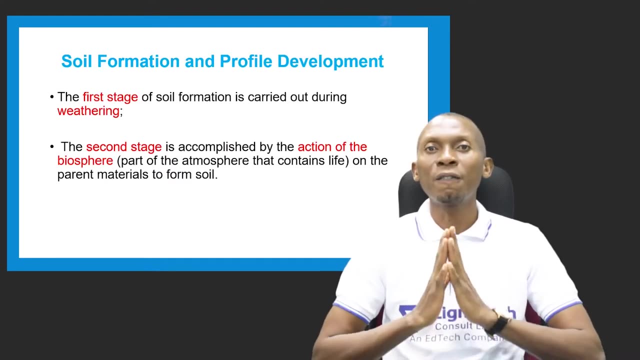 profile. So as you go further, understand what the soil profile is, which shows distinct layers of soil. but as we move forward, I'll talk about that Now. let's look at soil formation and profile development. Here we know that the first stage of soil formation has to do. 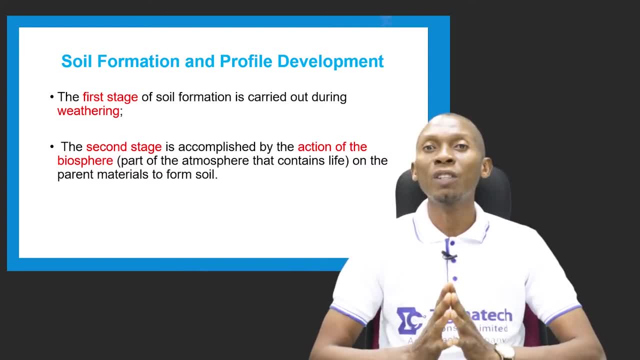 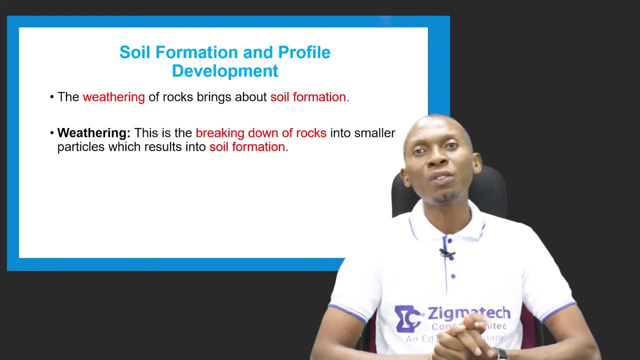 with weathering, while the second stage has to do with the action of the biosphere, which has to do with the living part, or the part of the earth that contains life. Now, weathering has to do with the breaking down of rocks to form soil, and when these rocks are broken down into tiny pieces, the soil is. 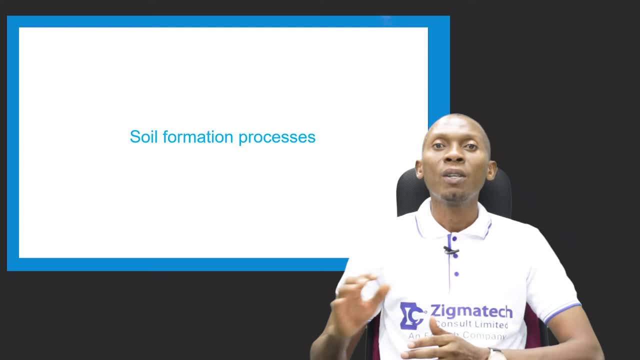 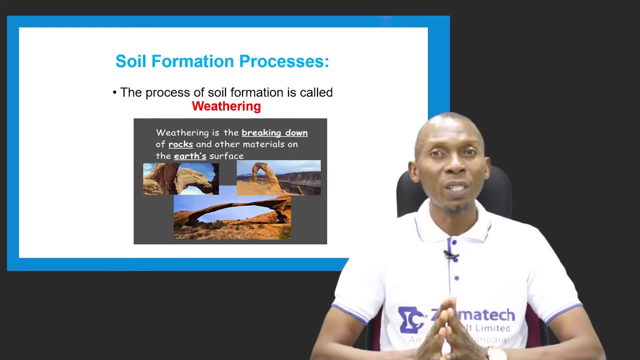 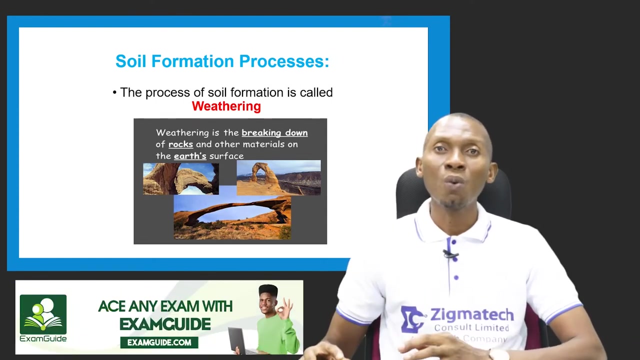 eventually formed after a long time. So let's look at, still on soil formation processes. I've defined earlier on that weathering is the process of soil formation. So the process by which rocks break down to form soil is called weathering. So that's the first stage of soil formation and under this 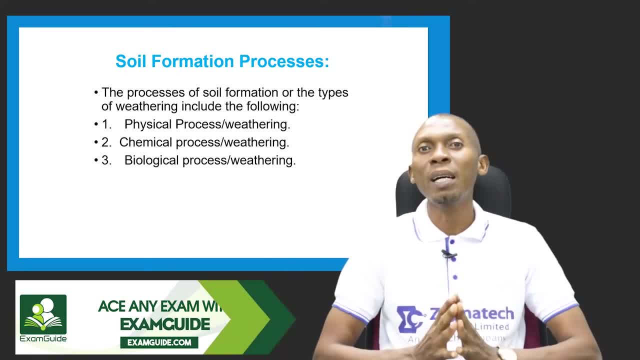 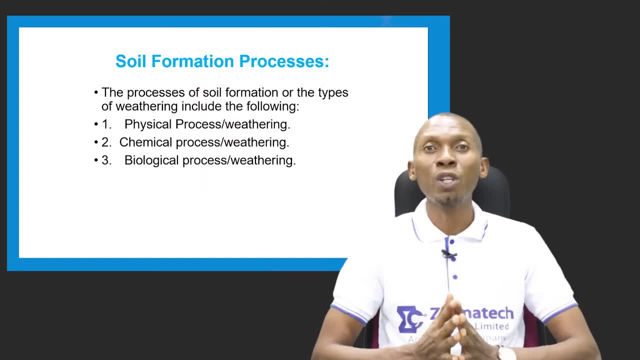 subtopic which has to do with weathering. we're going to look at three types of weathering. We have the physical weathering, or physical process by which rocks are broken down or by which soil is formed. We also have the chemical process of chemical weathering, That's the chemical process by which rocks are. 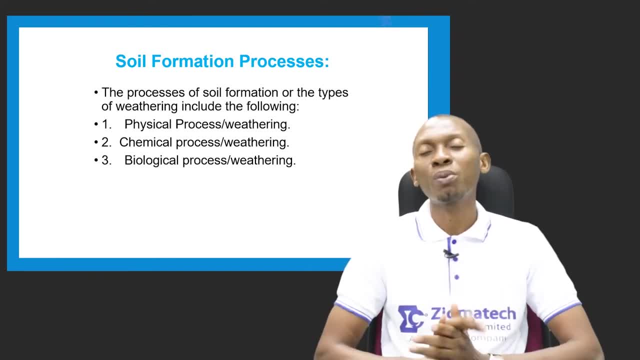 broken down to form soil. We also have the biological process process by which rocks are broken down to form soil and you can see I'm stating biological process or biological weathering, because weathering has to do with the breaking down of rocks to form soil. So, starting with the physical, 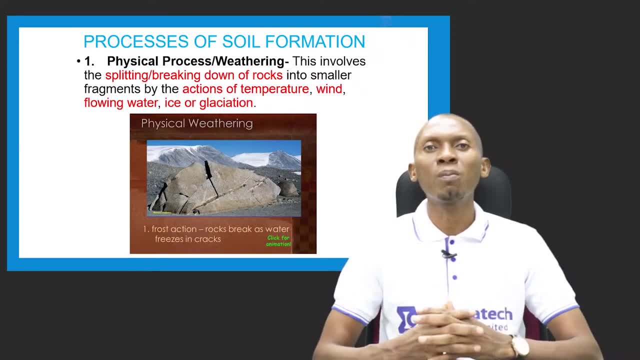 process of weathering. Now this has to do with the rocks being splitted into fragments as a result of the action of climate or things like temperature, wind, flame, water, ice or glaciation, So ice is also known as glaciation. Now this factors, or can? 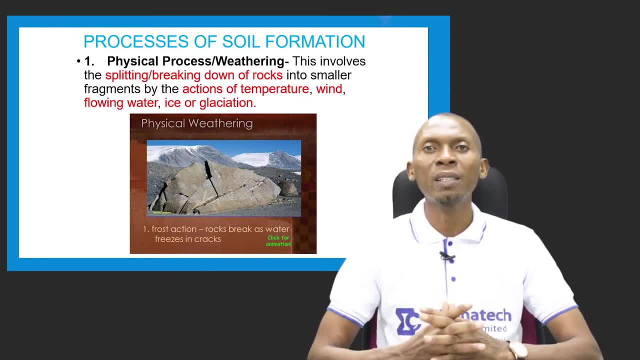 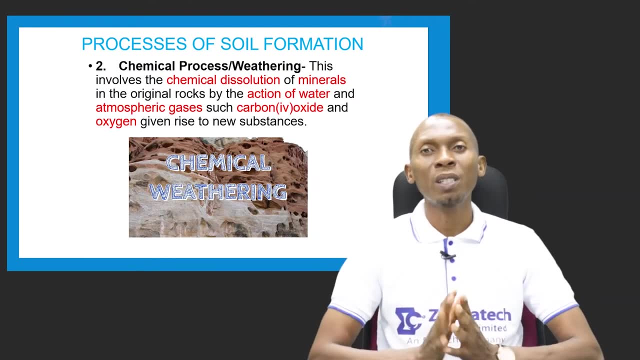 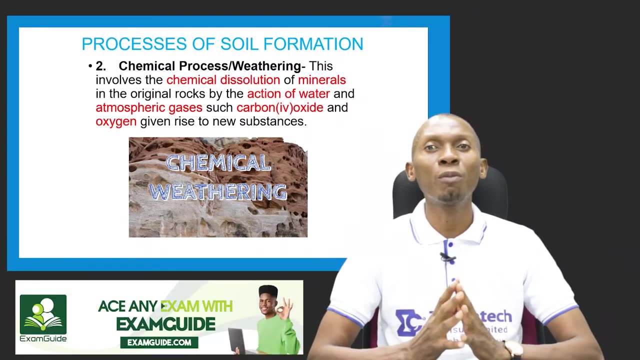 cause rock to break down or disintegrate, and once this takes place, it's called physical weathering. We also have chemical process of chemical weathering We have. this involves the dissolution of minerals. Now rocks are made up of minerals and once this minerals get in touch or in contact with water and atmospheric gases, such as 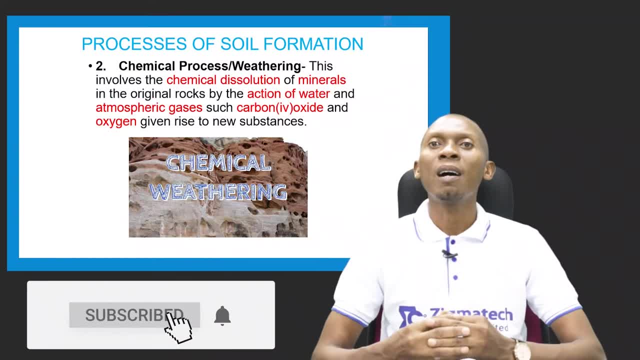 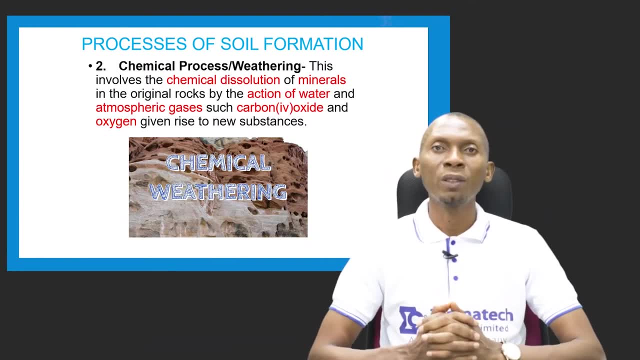 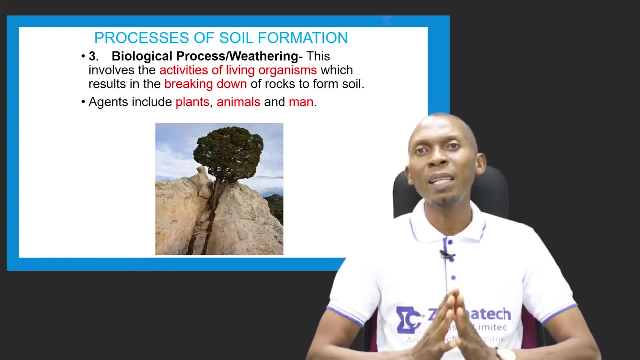 carbon dioxide and oxygen, new substances are formed and, as a result of this, weathering takes place, which is called chemical weathering. We have the biological process, or weathering. Now biological, here we're looking at living organisms. Now this living organisms, their activities, probably their burrowing. 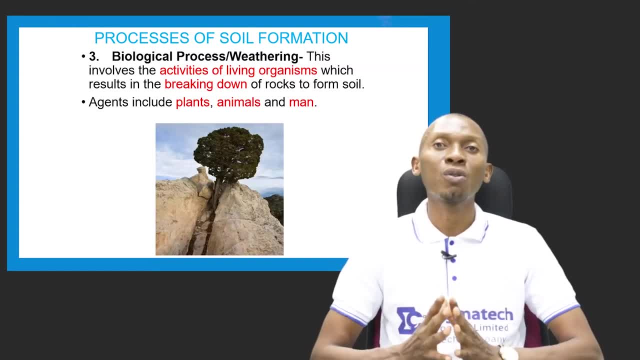 activities can cause these rocks to break down to form soil, and here this living organisms refer to plants, animals and man. This picture helps us to see how that tree has been able to cause their rock to split into two and eventually cause it to disintegrate to form soil. So the processes here we've talked about the 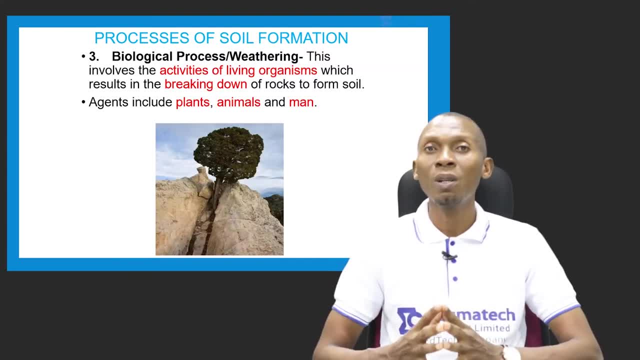 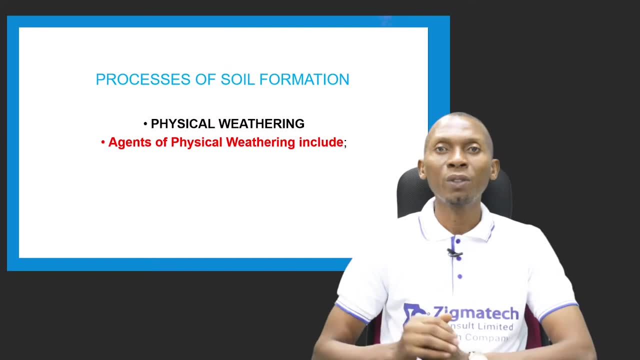 chemical process or chemical weathering. we've talked about the physical process of physical weathering. we also talked about the biological process, which is also called biological weathering. Now let's look at the agents of these various types of weathering. We're going to look at the agents of physical weathering. we'll also look at the agents of 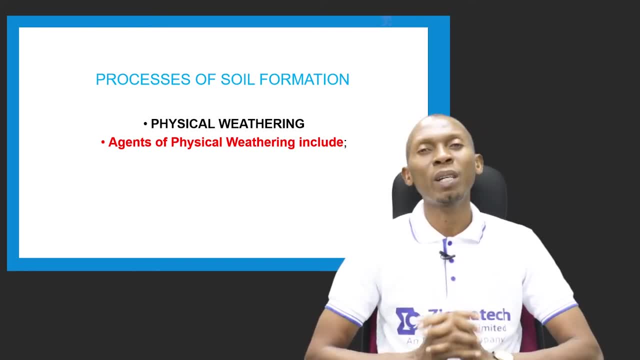 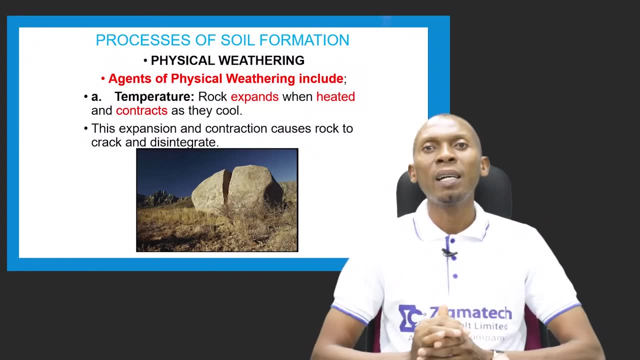 chemical weathering, and we'll also look at the agents of biological weathering. Starting with the agents of physical weathering. we have temperature as an agent, and how does temperature cause physical weathering to take place? Remember, weathering has to do with the breaking down of 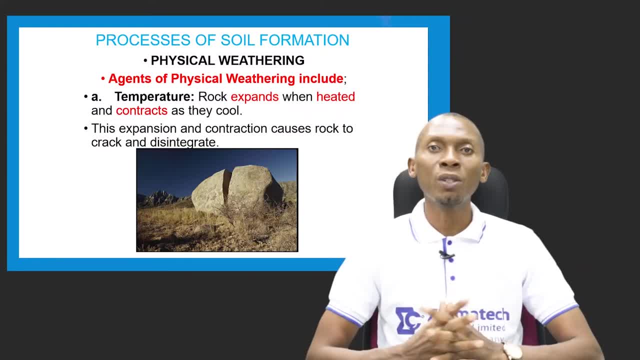 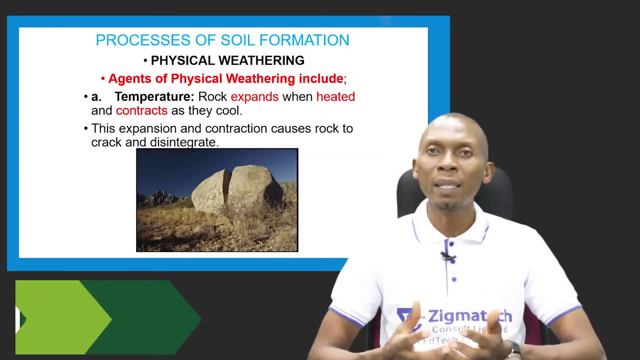 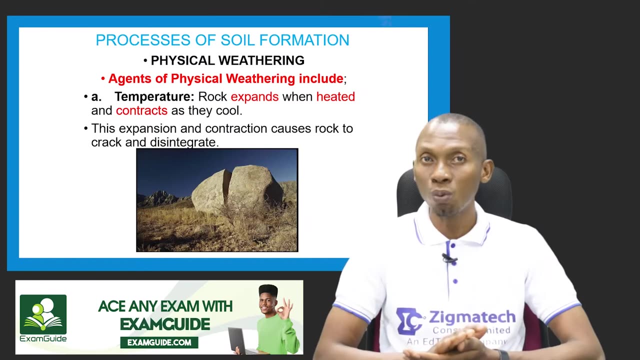 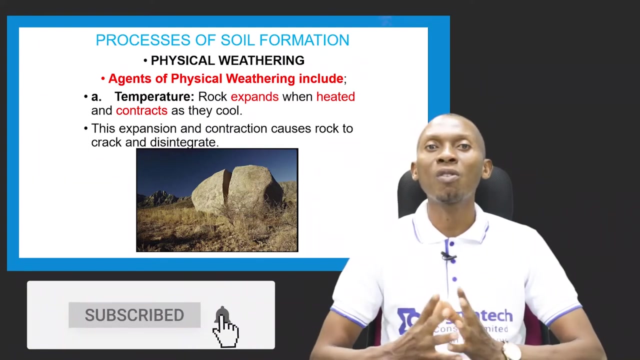 rocks to form soil. Now, temperature it has to do with the degree of hotness or coldness. In this case, it causes rocks to expand when heated, and these rocks also contract when the rocks get cold. So this continuous expansion and contraction over time will now cause the rocks to crack. 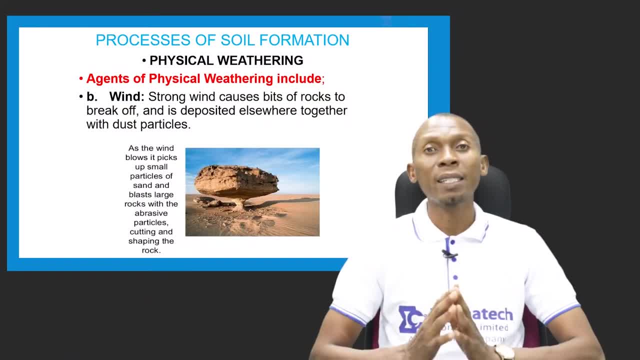 and eventually die, disintegrates. So our focus here now is how the agents of physical weathering act on the rocks to cause it to break down or disintegrate. We have wind as another physical agent or agent of physical weathering. Now strong winds can cause. 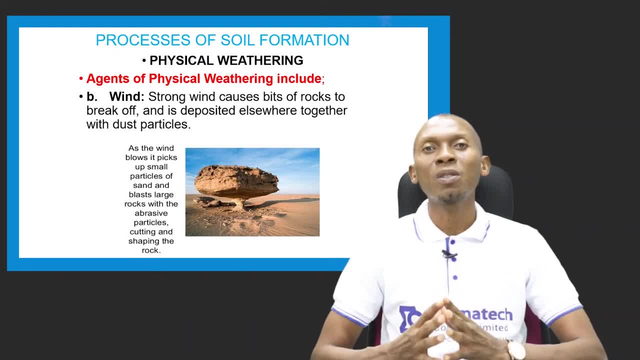 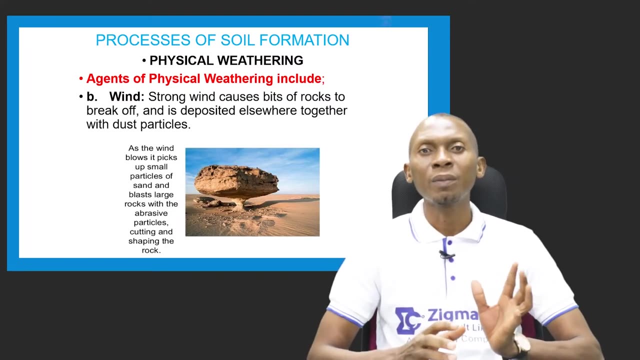 bits of rocks to break off, and these rocks, these bits, are eventually deposited elsewhere together with soil particles. So as the wind blows, it picks up the soil particles of sand and keeps on blasting the larger rocks with these particles, which will eventually lead to the disintegration of the rocks to form soil. 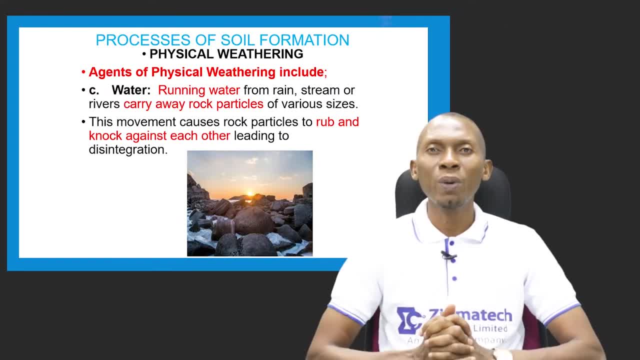 We have water as another agent of physical weathering. Now, here, while we're, fame is referring to running water from rain or streams or rivers, which can carry away rock particles of various sizes. and as these rock particles are moving, they begin to rub and knock against each other, and that impact will now cause the rocks to break or 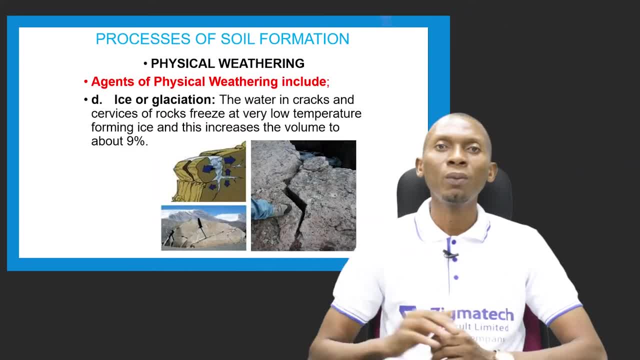 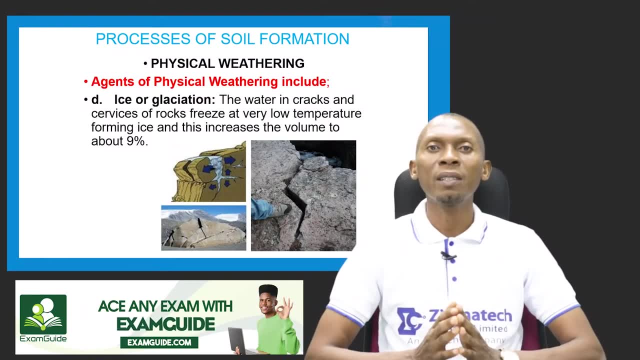 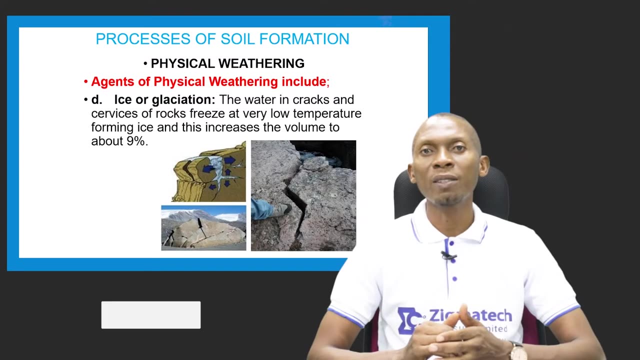 disintegrate to form soil, we have ice or glaciation. now, in this case, you can see that the cracks or crevices that are in rocks. water could then get filled into those cracks or crevices and as this cross of this, water freezes at low temperature, ice is formed, and once water freezes at that low, 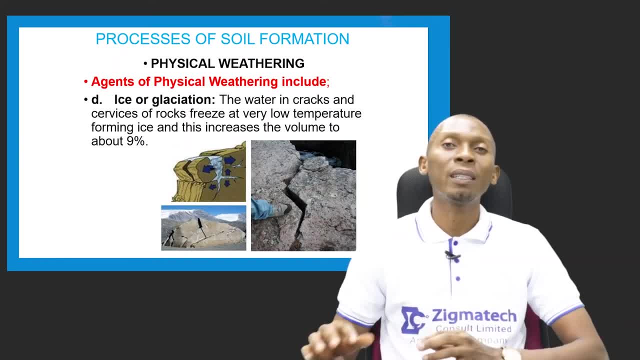 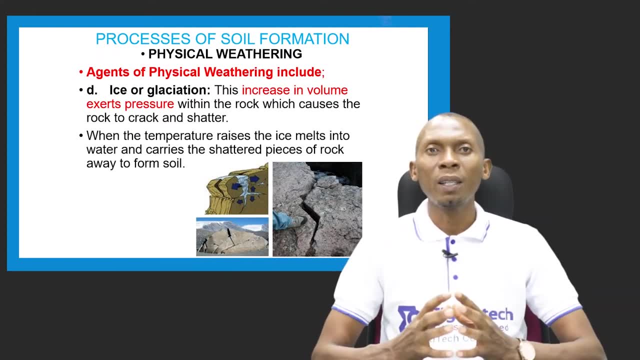 temperature and ice is formed, the volume increases to about nine percent now. as the volume increases, it exerts pressure. pressure is now exerted within the rocks and as a result of that, the rock will begin to crack and eventually shatter. so when the temperature rises, the ice will now melt, and once it melts, the water will now carry the shattered. 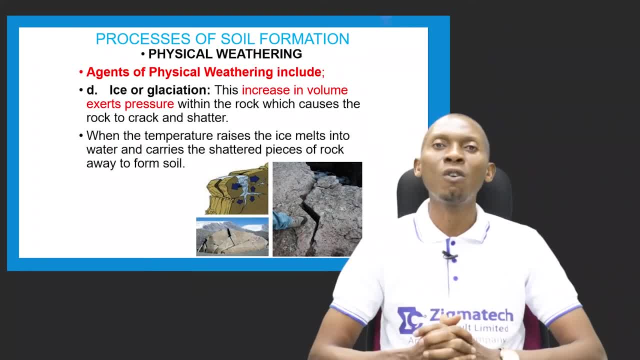 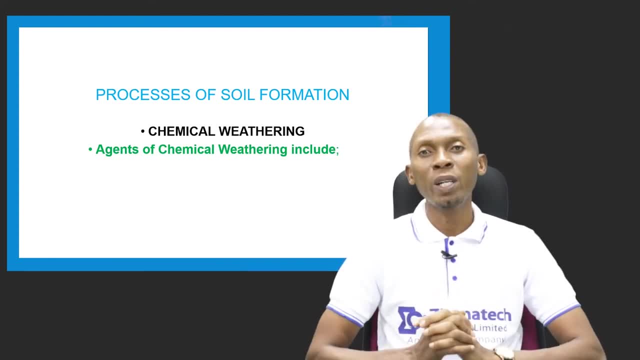 pieces of the rock away and eventually form soil. let's take a look at chemical red ring, now the agents of chemical weathering. so we will get to understand how these agents of chemical red ring lead to the breaking down or disintegration of rocks to form soil. now these agents of chemical 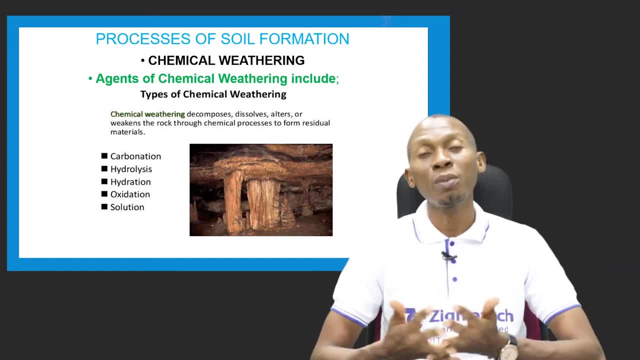 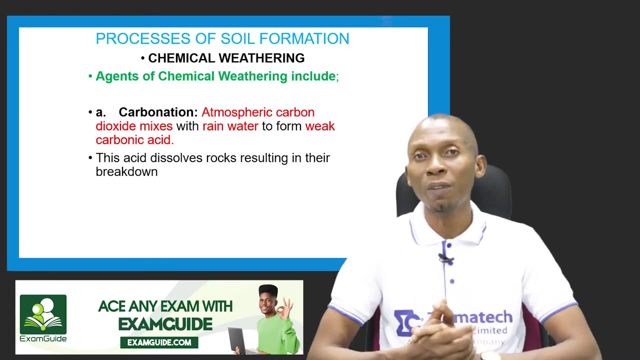 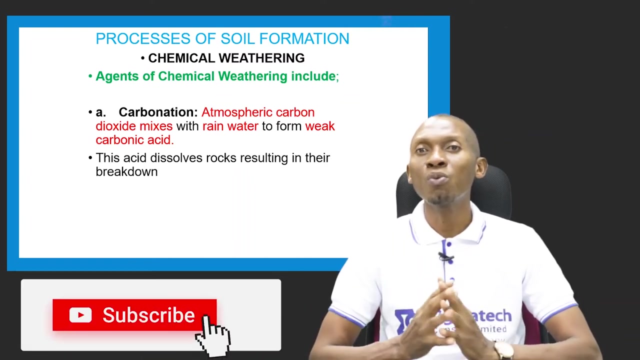 weathering include carbonation, which can also be called types of chemical regments. they include carbonation, hydrolysis, hydration, oxidation and reduction, and we also have solution. so, starting with carbonation as an agent of chemical regimen or a type of chemical woman, here we're looking at carbon dioxide in the atmosphere, which now mixes with rain water. 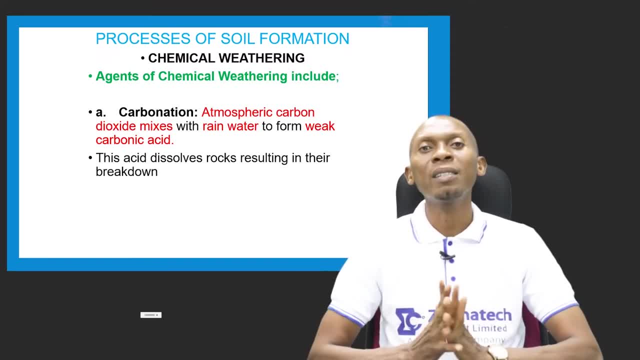 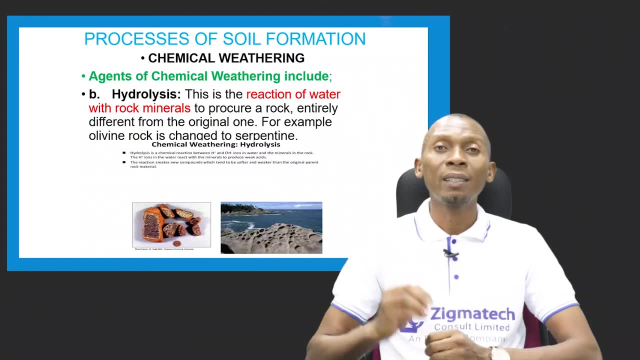 to form carbonic acids. now this carbonyl atoms, current acid acid isriminated with comorbid-3-derains, will cause rocks to break down and disintegrate. So that is carbonation as an agent of chemical origin. Now hydrolysis as an agent of chemical. 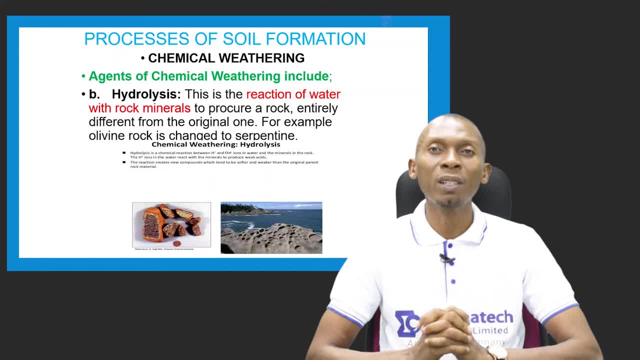 origin also has to do with the reaction of water with rock minerals, and this reaction leads to the procurement of a rock which is different from the original rock that existed. For example, we have a rock that is called olivine and once water gets in contact or reacts with the rock minerals, this olivine 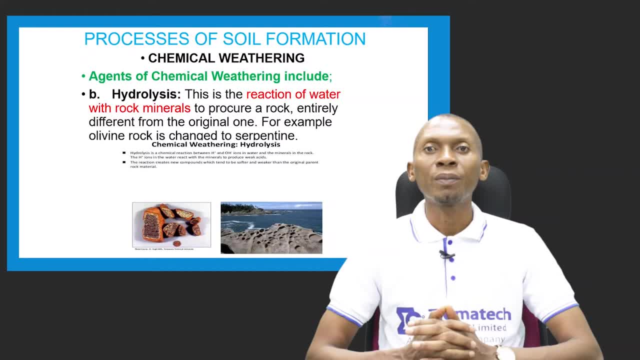 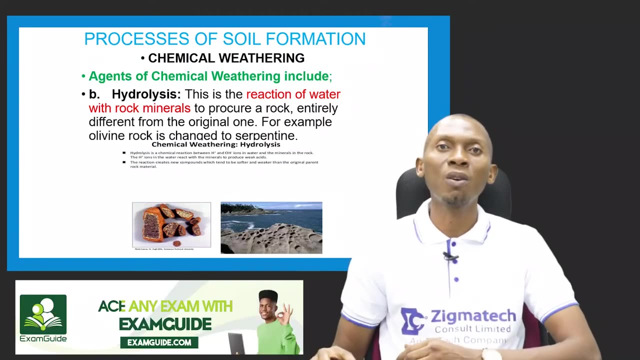 rock is changed to serpentine, which is usually softer and weaker than the original olivine rock, and this will eventually lead to the breaking down of disintegration of the rock. So this process is called hydrolysis. We have hydration Now. this also involves 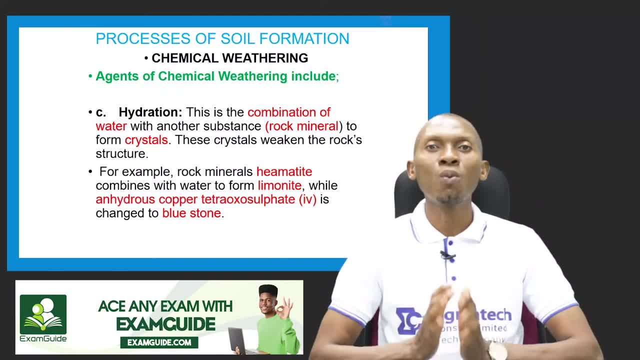 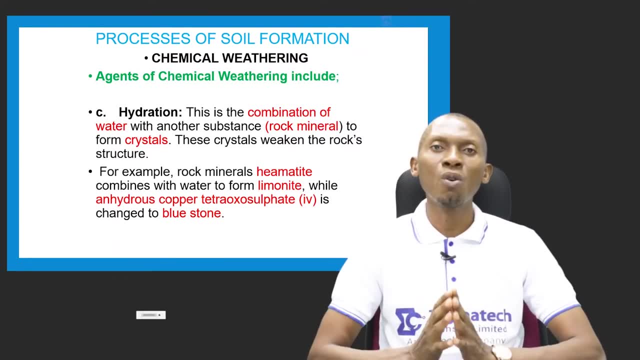 water and rock minerals. Now, in this case, the water combines with the rock minerals to form what is called crystals, and these crystals will now cause the rocks structure to get weakened, and once it's weakened, the rocks eventually disintegrate. Now an example here is hematite, which combines with water to 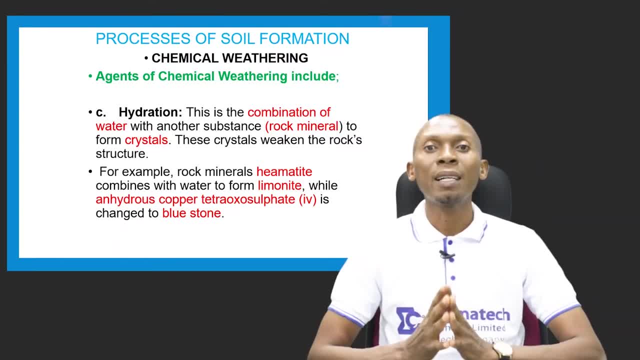 form limonites. And another example is anhydrous copper tetrahydrosulfate 4,, which now reacts with water to form what is called bluestone. So this is what is called hydration as a means of weathering, chemical weathering. 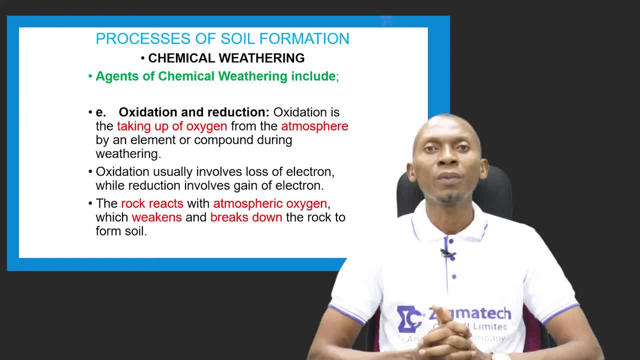 We have oxidation and reduction, because oxidation has to do with the taking up of oxygen from the atmosphere by an element or a compound during weathering, and oxidation has to do with the loss of electrons, while reduction has to do with the gain of electrons. 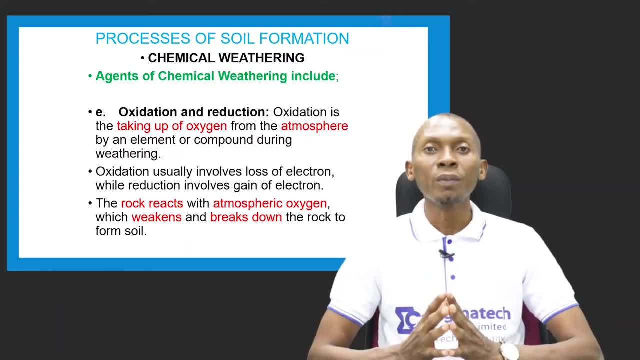 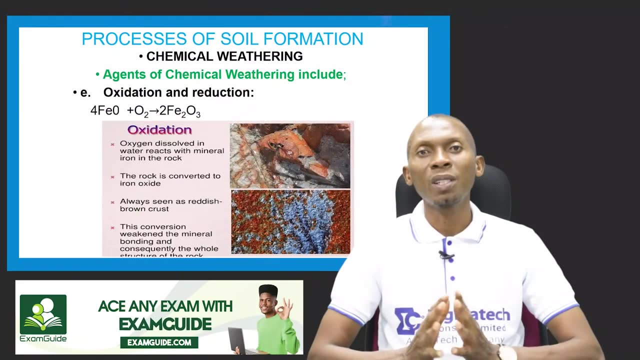 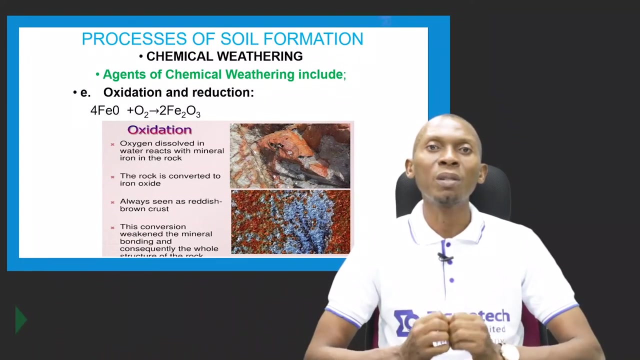 So once these rock minerals react with atmospheric oxygen, they get weakened and eventually the rocks break down to form salt. So this also still explains oxidation and reduction. So you can see if oxygen reacts with a mineral ion. for example, you find out that the rock mineral is now converted to iron oxide, which is now seen as a reddish-brown crust. 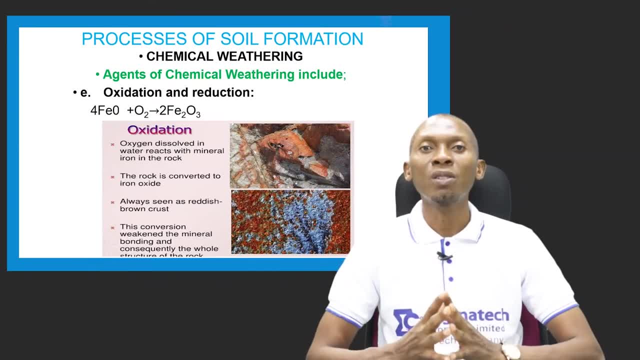 Now this conversion will now eventually cause the rocks to disintegrate. Still on oxidation and reduction you can see iron. when oxygen which is dissolved in water reacts with a mineral ion in the rock, This now converts that mineral ion into iron oxide, which can now be seen as a reddish-brown crust. 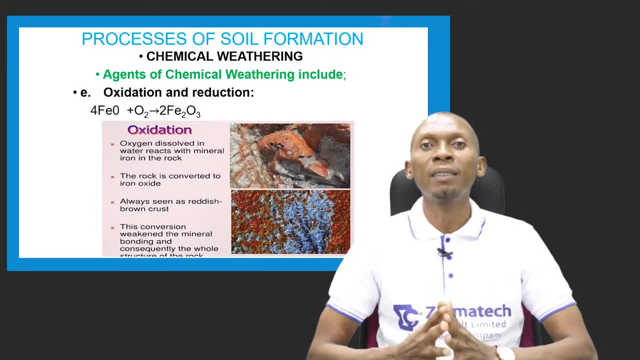 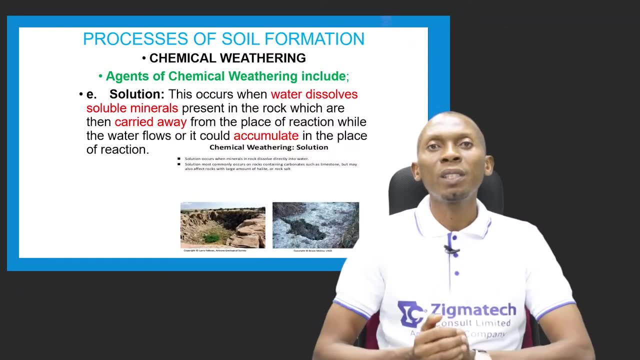 And this conversion weakens the bonding and you can see that it will eventually lead to the disintegration of the rock. Solution is another chemical or agent of chemical weathering. Now this has to do with water as well. Water is a very important element in the process. 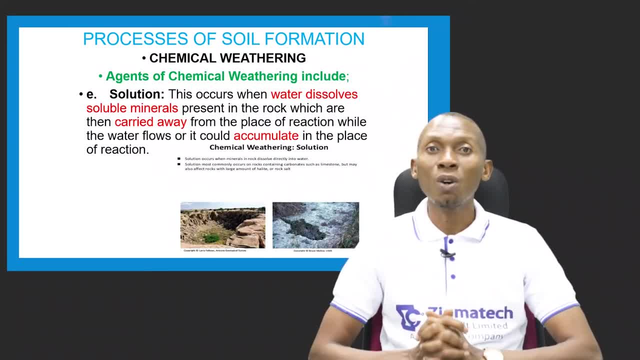 Solution is another chemical or agent of chemical weathering. Now this has to do with water as well. Water now dissolves soluble minerals that are present in rocks And, as a result of this dissolving of these soluble minerals, the rocks, they are carried away from the place of reaction while the water flows. 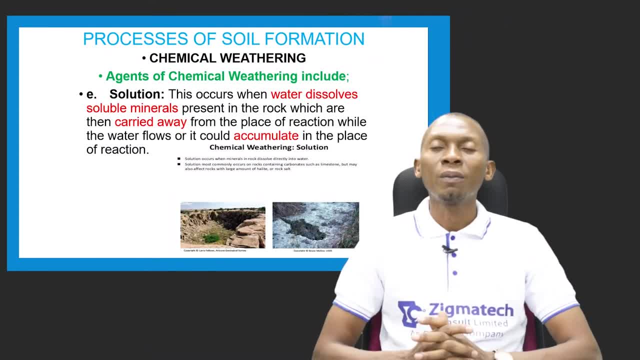 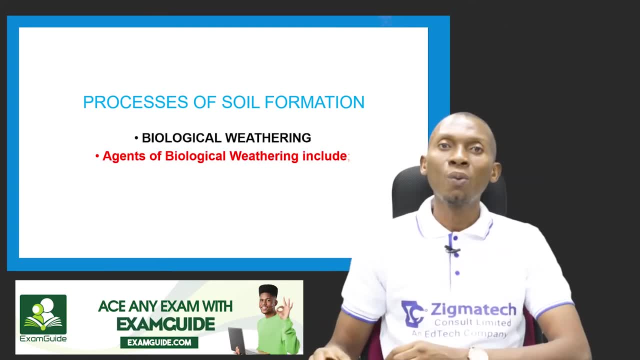 or they could be accumulated in the place of reaction. Let's look at biological weathering, That's, the agents of biological weathering. Now, the first agent we have here is what is called micro-organisms. Now, how do these micro-organisms 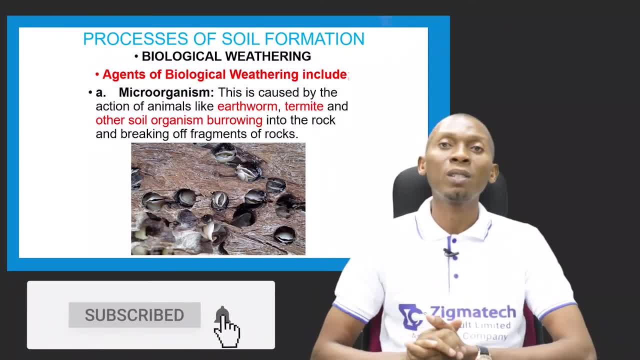 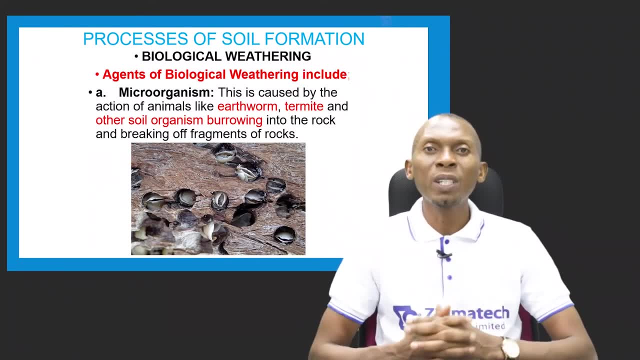 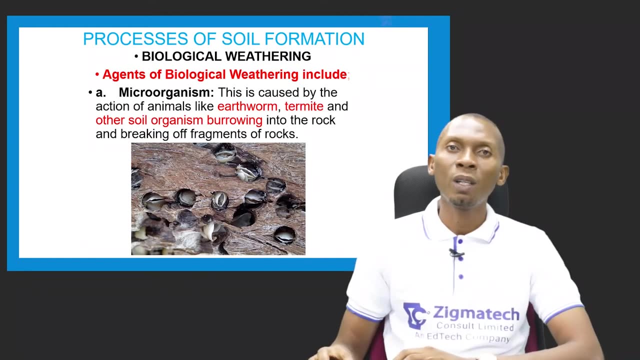 How do these micro-organisms cause weathering of rocks? Examples of these micro-organisms include earthworms, termites and some other soil organisms that could burrow into these rocks, And these burrowing activities can cause the breaking of fragments of rocks, which eventually will form soil. 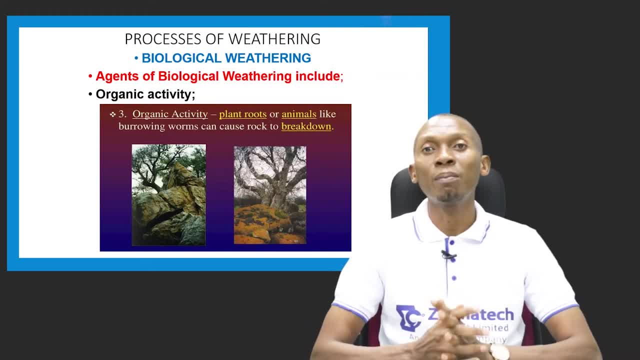 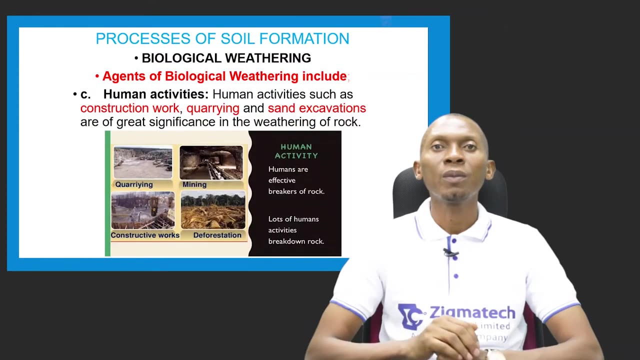 We have organic activities Now. this has to do with plant roots. We can see that these plant roots can eventually, Or animals like Burrowing worms can cause these rocks to break down and this will eventually lead to soil formation. Human activities is another agent of biological weathering. 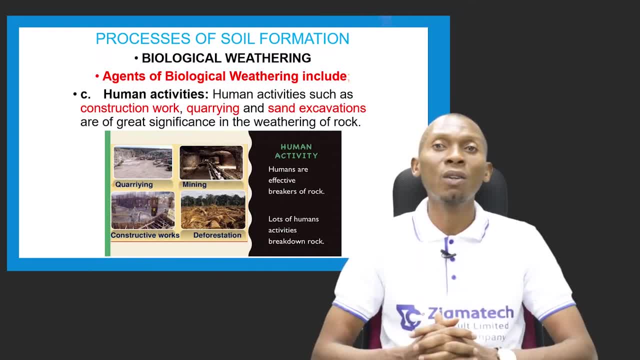 Now, how does human activities cause weathering? You can see construction works, quarry, which has to do with the breaking of rocks, you know, And also sand excavation can also have, or do also have, great significance in the Broken down of rocks. 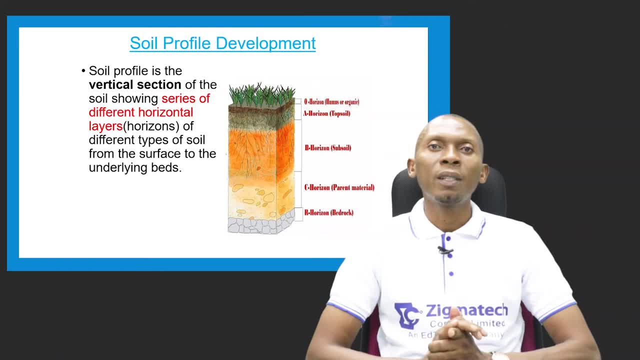 Now let's look at the soil profile. Now, soil profiles have to do with a vertical section of the soil which shows series of different horizontal layers Of the soil, Or different horizons of the soil, of different types of soil, From the surface to the underlying beds of the soil. 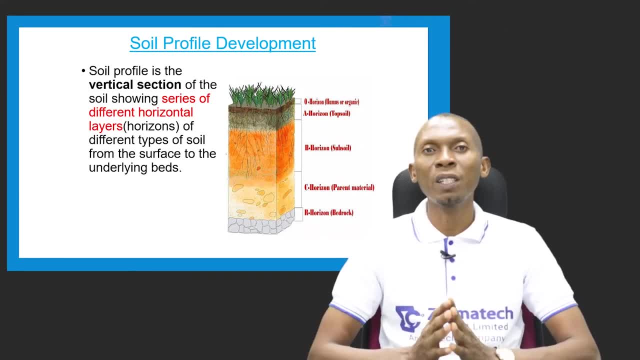 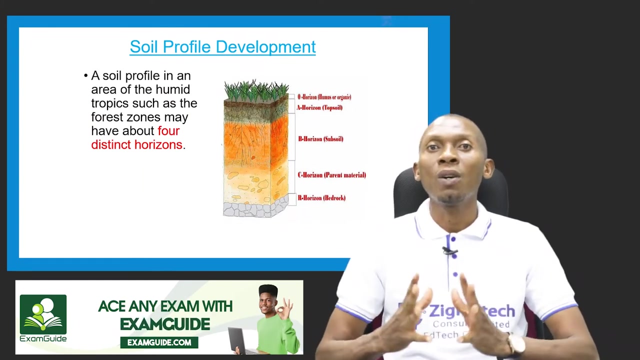 So the soil profile has to do with the vertical sections Of the soil. vertical section Vertical means from top to the bottom, So you can see showing the different horizons or different layers or horizontal layers of different types of soil that can be seen. So that's what the soil profile is Now in humid areas you can see. 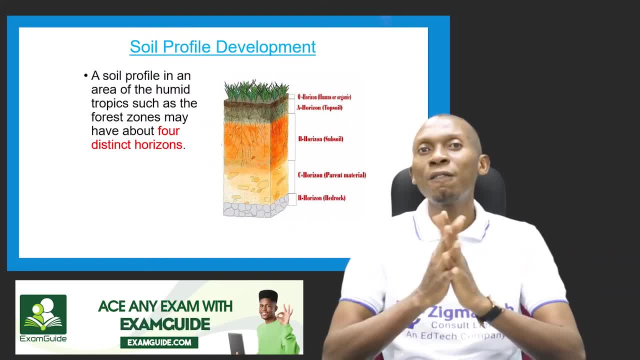 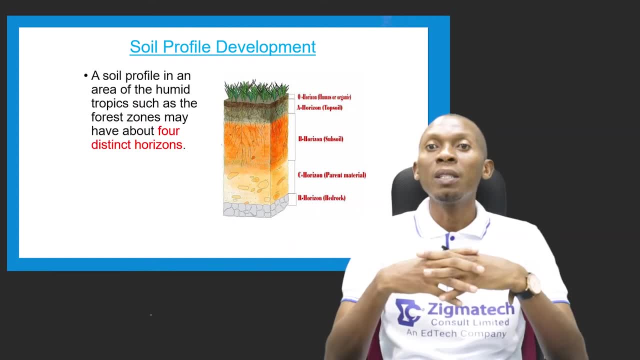 the soil profile, such as the forest zone. You can see the soil profile has four distinct horizons where we have the A-horizon, the B-horizon, the C-horizon, the D-horizon or the R-horizon in some cases. So the A-horizon is the topsoil, the B-horizon is the subsoil. 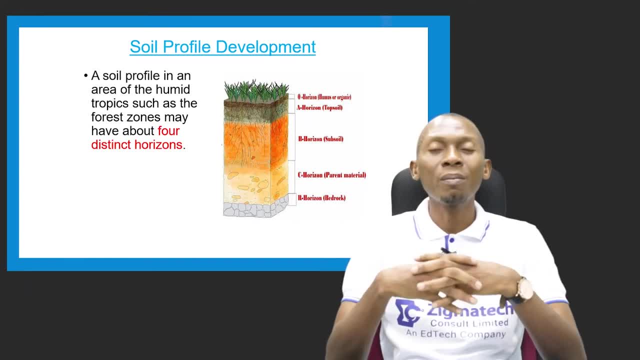 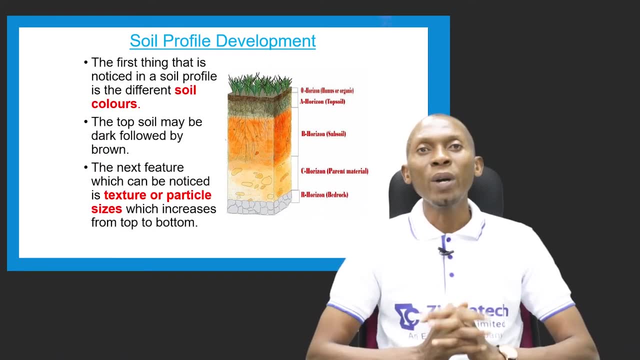 the C-horizon is the parent material and the D-horizon is the bedrock. Now, these are the four distinct horizons that are seen in the soil profile. Now, when you look at the soil profile, the first thing you will observe in the soil profile are the different soil. 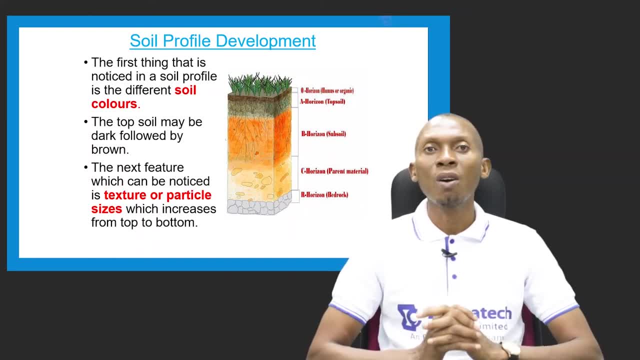 columns. So from that picture you can see that there are different soil columns. So the topsoil is usually dark, followed by brown and so on. Then you can also see another feature that is observed, or observed in the soil profile has to do with the texture or the particle. 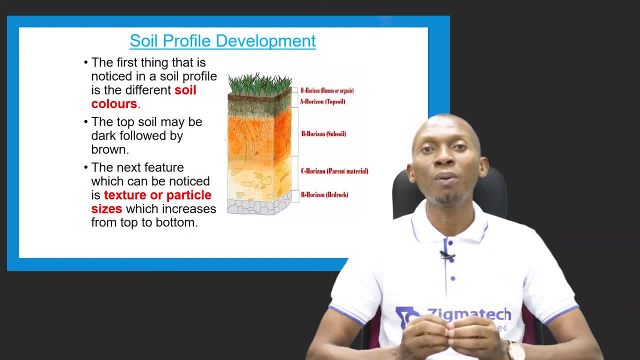 size, which also increases from the top. That increases its size from the top of the soil profile to the bottom of the soil profile. So as you go down to the bottom of the soil profile you can see that you have a larger size of the soil. 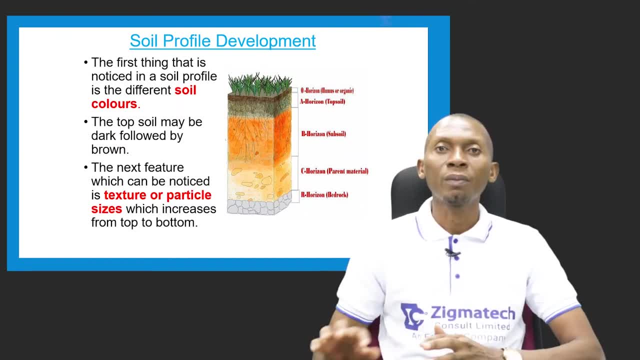 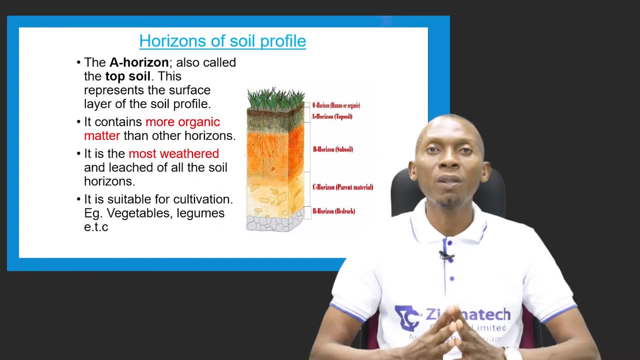 This is the surface of the soil. Now, starting with the A-horizon. remember we were talking about the A-horizon, the B-horizon, the C-horizon and the D-horizon. The A-horizon. 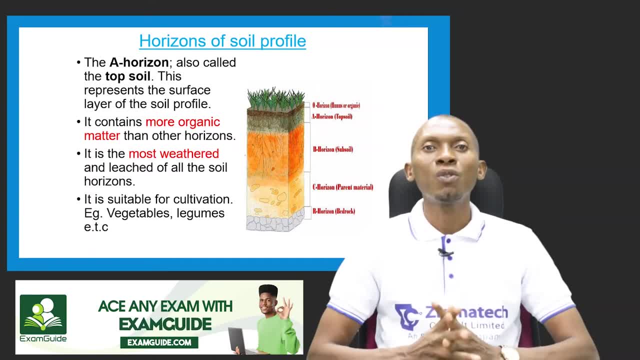 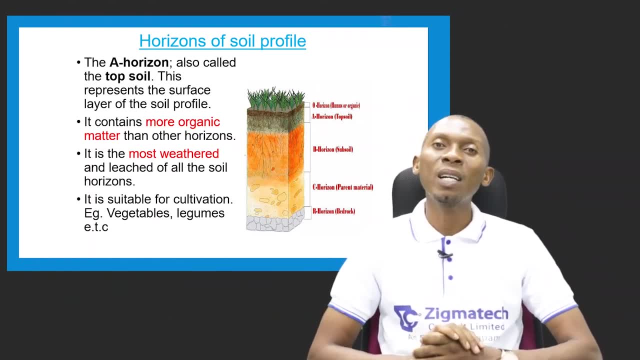 is also called the topsoil. Now this represents the surface layer of the soil profile. Now, this layer contains more organic matter than any other horizon and it's also the most organic matter, also the most weathered horizon and the most leached. Now, leaching has to do with the washing. 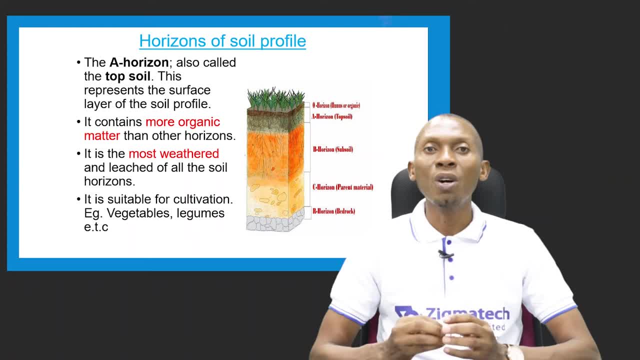 away of nutrients beyond the reach of the roots of plants. So it's the most weathered and it is the most leached of all the horizons and it's suitable for the cultivation of certain crops like vegetables, legumes. those are crops that are not deep rooted, So they are. 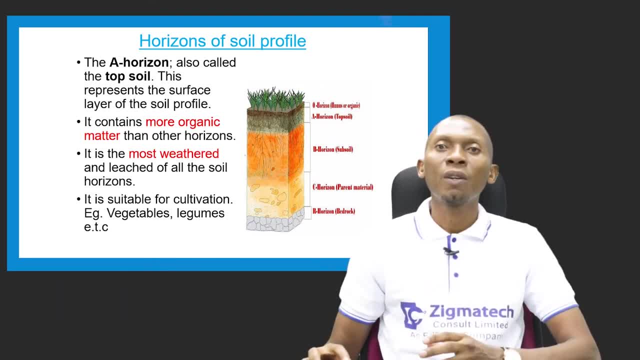 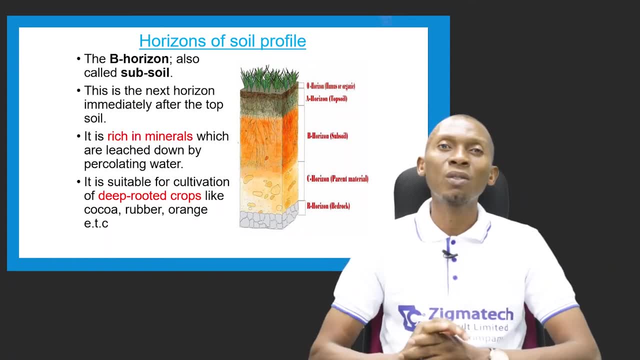 shallow rooted crops, So it's suitable for such crops as are the A horizon, While the B horizon is also known as the subsoil and is the next horizon after the A horizon, which contains the topsoil. Now it's also rich in minerals, which are leached down to the 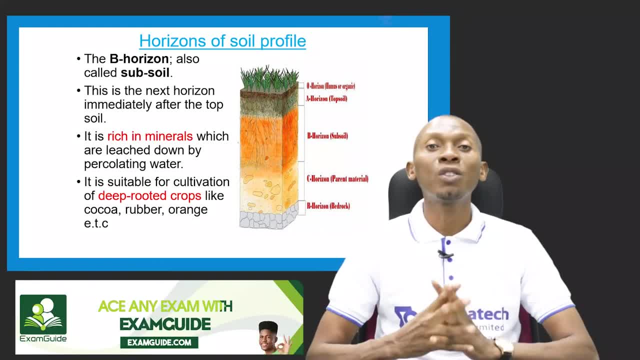 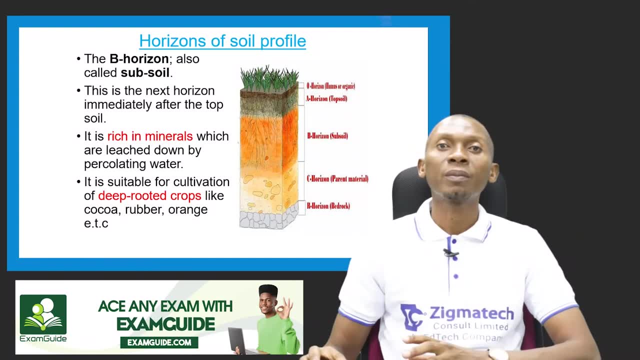 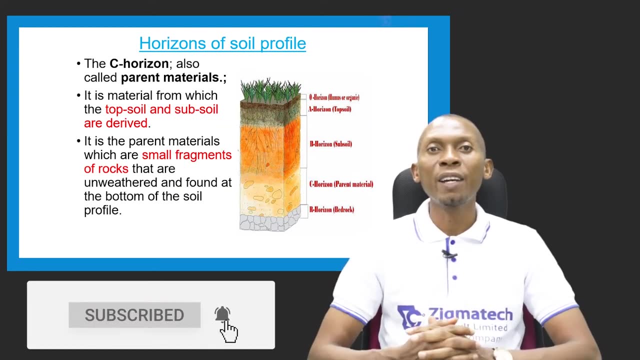 bottom by percolating water, And it's suitable for deep rooted crops like cocoa, rubber, orange tree crops as well. We have the C horizon, which is called the parent material. Now, this is derived from the topsoil and the sorry it is materials from the topsoil, from. 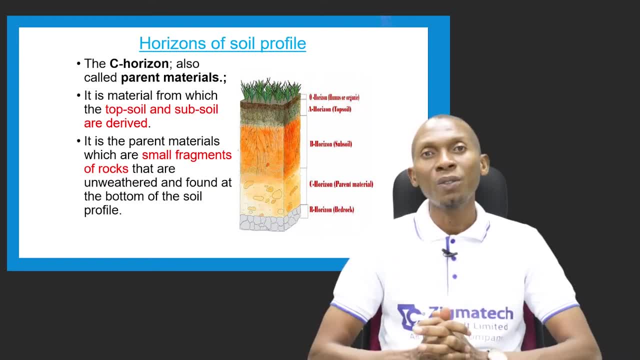 where the topsoil and the subsoil are derived. So the C horizon comes from the topsoil and the subsoil are derived. So the C horizon comes from the topsoil and the subsoil are derived. So the C horizon is where the topsoil, where the materials that are for the topsoil. 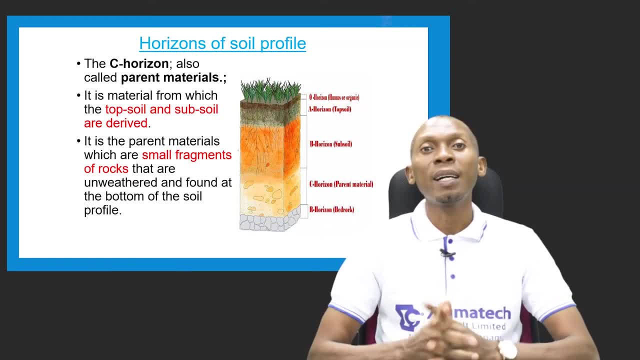 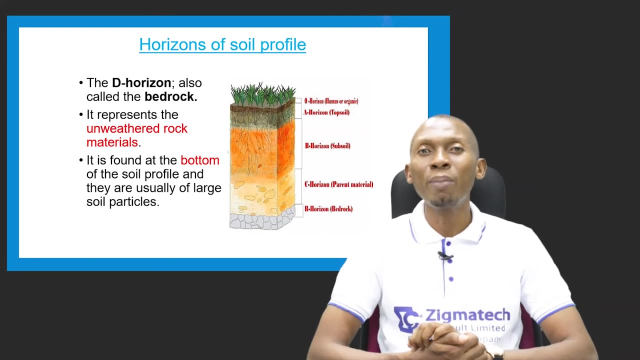 and the subsoil have been derived or are derived from. Now it's the parent material, which are small fragments of rocks, And these small fragments of rocks are unweathered and they are found at the bottom of the profile. We have the D horizon, which is called the bed. 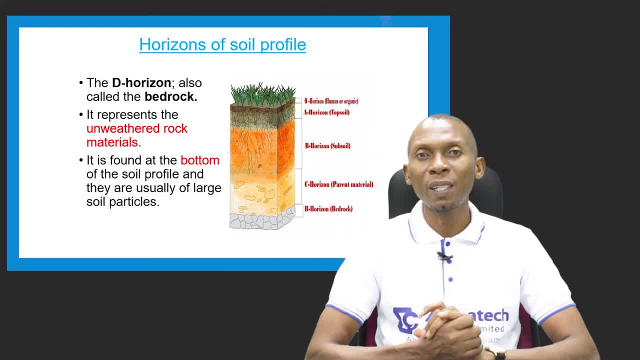 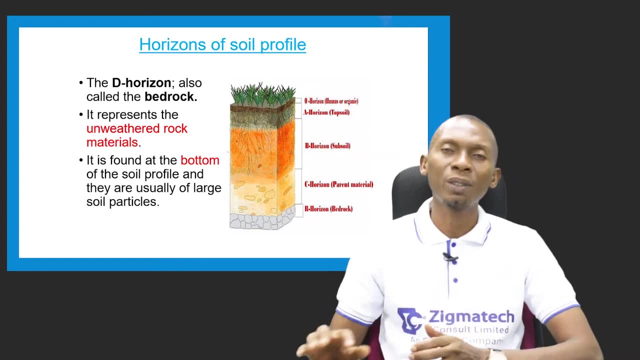 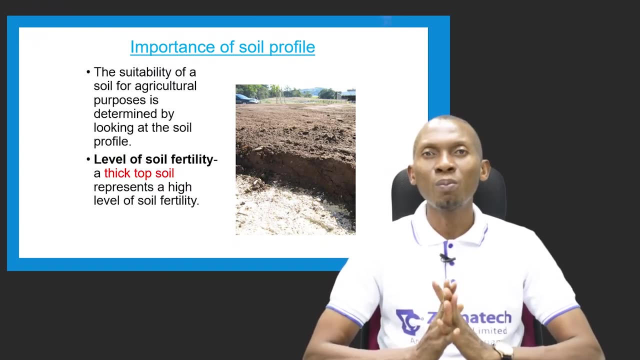 rock. It also represents unweathered rock materials and is found at the bottom of the soil profile. Now the C horizon usually contains large soil particles. Let's look at the importance of the soil profile. Why is the soil profile, or knowledge about the soil profile, important? Now it's a suitable or the suitability of the soil for agricultural. 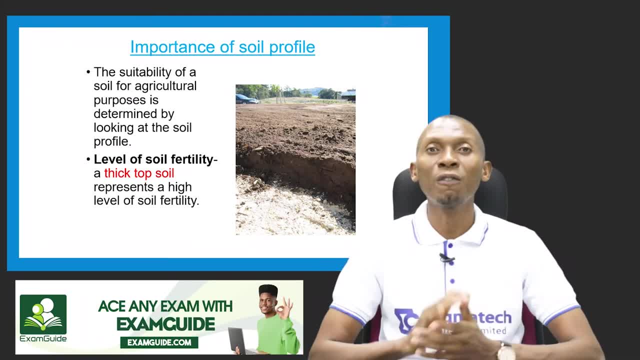 purpose is determined by looking at the soil profile. So if you want to know whether a soil is suitable for agricultural purposes, you need to take a look at the soil profile. One of the importance of the soil profile is that it helps us to know the level of soil. 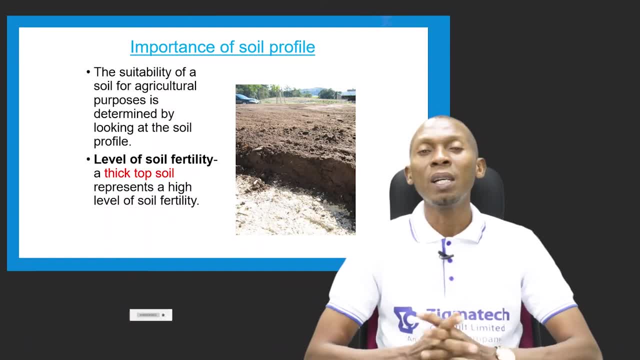 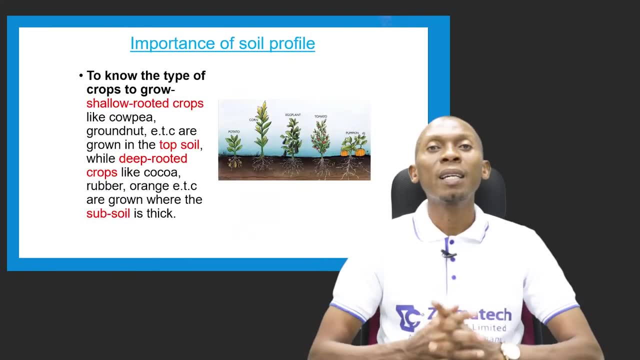 fertility. So once you have a thick topsoil, such topsoil represents a high level of soil fertility. It can also help us to know the type of crops to grow. Remember, I talked about shallow-rooted crops and I talked about deep-rooted crops, So you 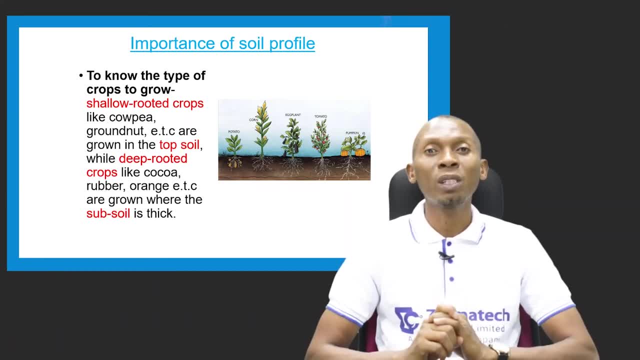 can see that shallow-rooted crops grow at the topsoil, while deep-rooted, shallow-rooted crops, like, of course, granite, maize and even lower microplastics, tomarckaa samples And, of course, low-temperature food. It's an area that are growing in naturals, for example. 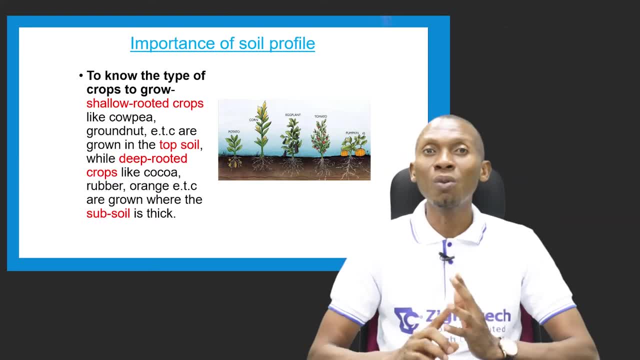 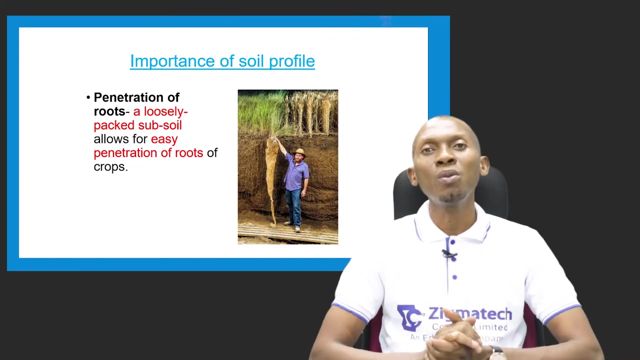 cowpea, you know, grow vegetables. They grow on the top soil, while deep-rooted crops, like our tree crops- oranges, lemon, rubber, cocoa- do grow on the soft soil, which has to do with the bee horizon. So now we can also know about the penetration of roots. 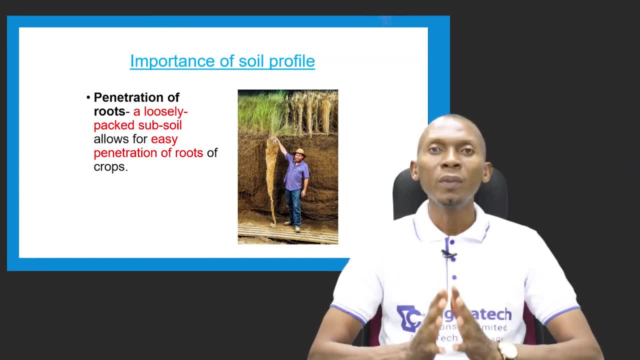 through the soil profile. Now, a soft soil or a loosely packed soft soil will always allow for easy penetration of roots of our crops. So the roots of our crops, if the soft soil which is after the top soil, that's the bee horizon, is loosely. 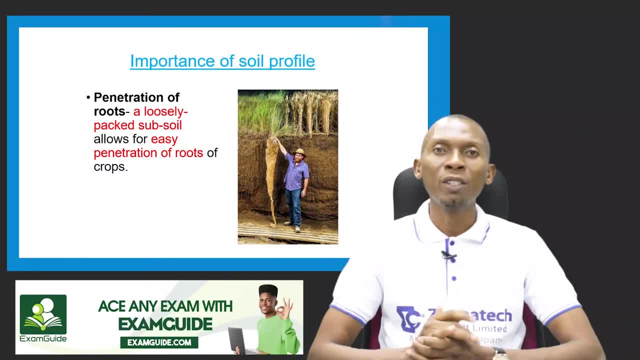 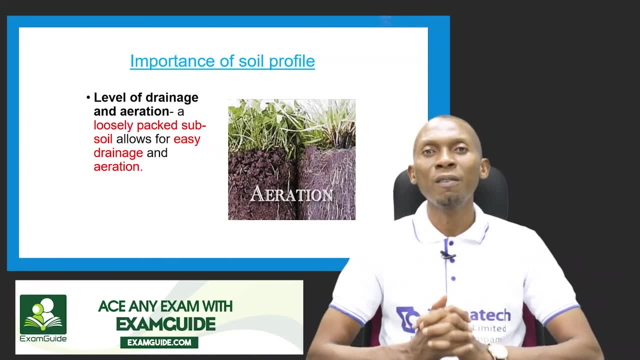 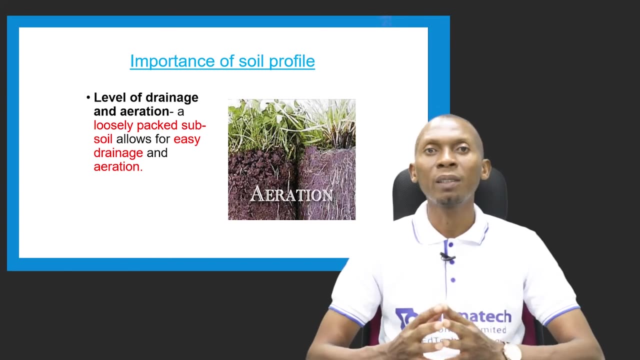 packed, the roots of our crops can easily penetrate. So that's another importance of the soil profile. We also have level of drainage and aeration, because drainage has to do with the movement of water within the pore spaces of our soil particles and aeration also has to do with movement of. 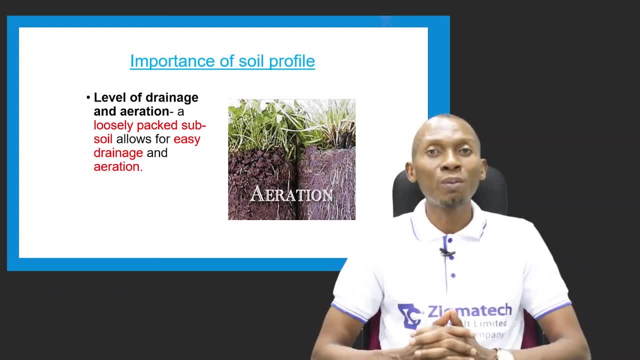 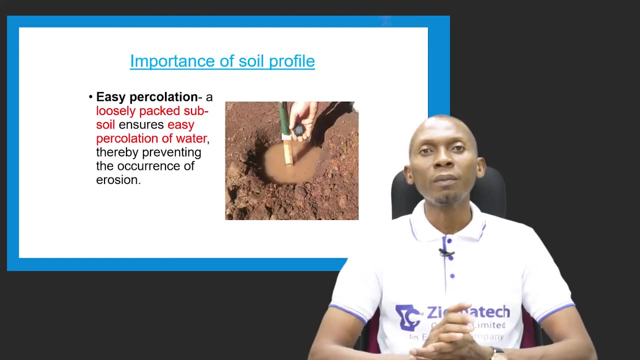 air. So a loosely packed soft soil will also ensure that there's easy drainage and also aeration. So we're able to know the level of drainage and aeration as a result of our soil profile. knowledge of the soil profile. Another importance is easy percolation. If the soft soil is loosely packed, the water 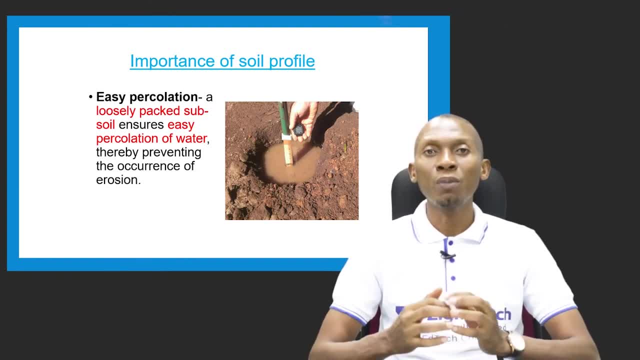 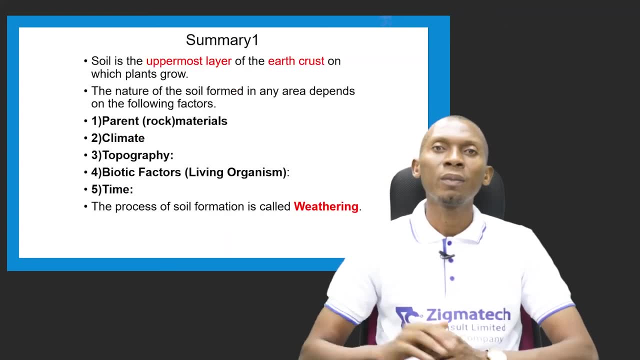 there will be easy percolation of water, which has to do with the absorption of water or the downward movement of water, and this will help to prevent erosion. Okay, we've learned so far quite a number of things, but let's just have a recap of what we've learned. 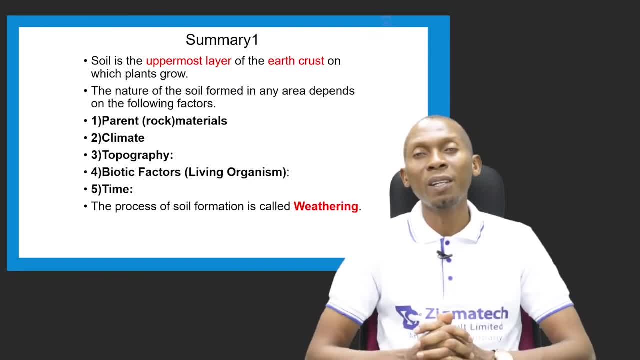 I started by defining soil. I said soil is the uppermost layer of the earth's crust on which plants grow, And the nature of soil formed in an area depends on some factors, and these factors include the parent material climate, such as temperature, water, wind. 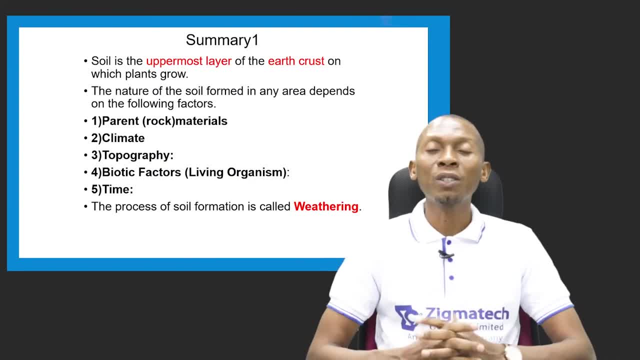 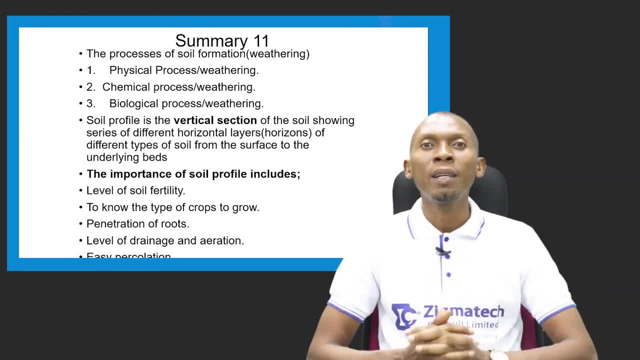 soil is the lower layer of the earth's crust. soil is the lower layer of the earth's crust formation, which has to do with weathering, And here we're looking at. we talked about physical process of physical weathering. We also talked about 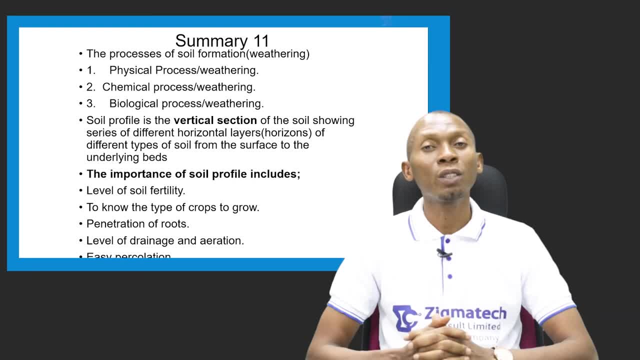 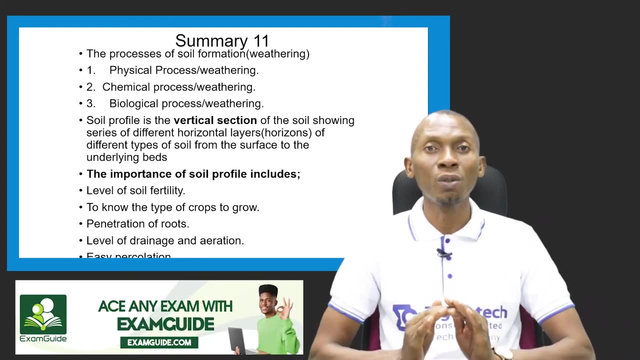 chemical process: chemical weathering. I also looked at biological process of biological weathering. We also defined soil profile as a vertical section of the soil showing the series of different horizontal layers or horizons of different types of soil, from the surface of the soil to the underlying beds. We 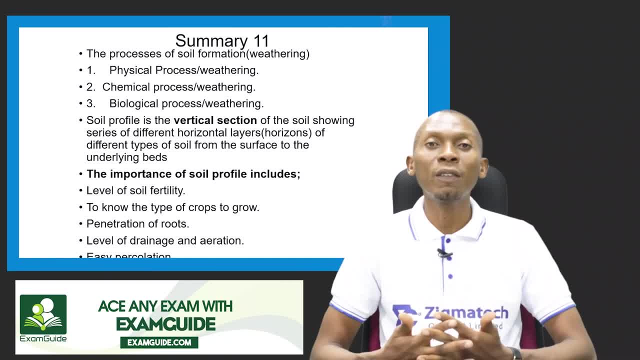 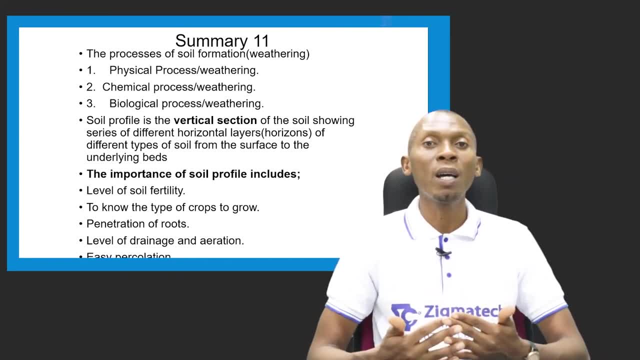 also looked at the importance of soil profile, which includes a level of soil fertility, helping one- the farmer, to know the level of soil fertility. also helping the farmer to know the type of crops to grow. also looking at the penetration of roots- we're talking about shallow rooted crops and deep rooted crops- and 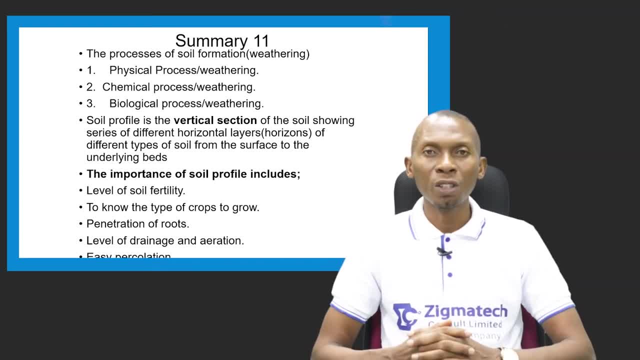 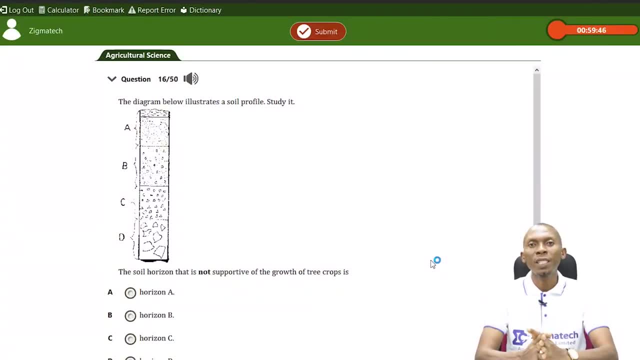 also the level of drainage and aeration. So let's take a look at some questions using the diagram below. illustrates the soil profile. We said we should study it Now. the soil that is not supportive of the growth of tree crops. horizon a- B option. horizon B: 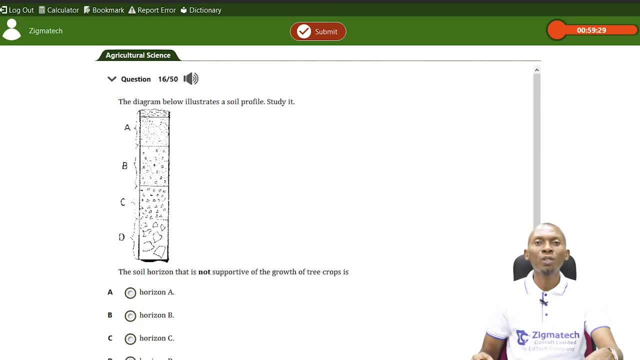 C option or is on D and D option. horizon D: the answer should be D option. that is, the bedrock and at that point, this integration of rock. the rocks are still very large and I've not been disintegrated. they have large particles. so the place that supports the growth of tree crops is the a horizon, B horizon and the C horizon? the answer is D. so which of the following agents is not associated with chemical weathering? so the agents are sort of chemical weathering. if you can remember, we talked about hydration, hydrolysis solution, oxidation reduction, carbonation. so a option here says oxidation, B option. 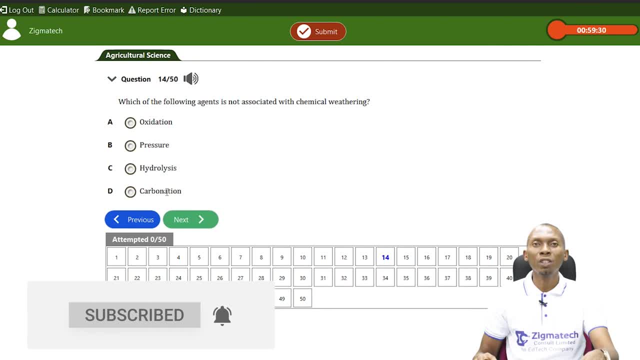 pressure, C option- hydrolysis. D option: carbonation. the answer here is pressure. so this question says: in chemical weathering of rocks, the equation this is iron oxide plus three molecules of water. with this water you can see we're talking about hydration, forming hydration hydrolysis of two molecules that is characterised by the one fact in which 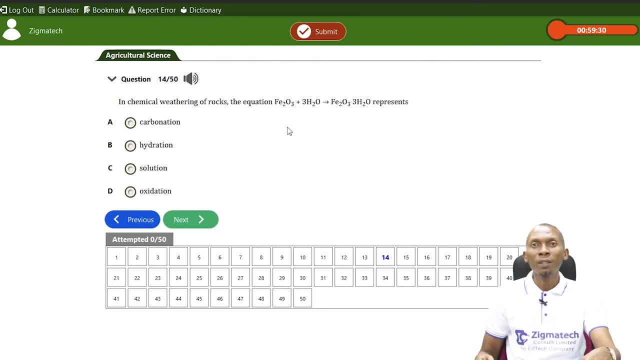 we can discuss. we're talking about circulating mineral water in this organic material called the hydrolysis was created by two refugee populations, people in the United States. the двигations that were fats felt horrible. we can pacing controversialuly with the question of all the very survival. relation between carbonate of the chemical, as how is Section? this equation represents a carbonation be hydration c solution diye audition. so the answer here is the opportunities to deflect the carbonation of insects. aroma is healthy, Kal Abraham is a global yield interest would. the answer here is alright. thanks, Rohokancia, would you like me the other half? so for the other half, you are a coholder with us today. hour to. 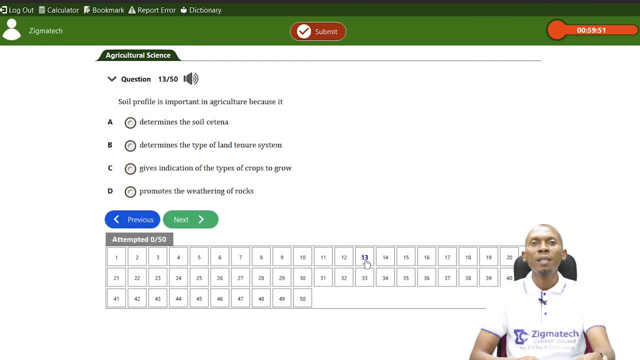 is important in agriculture because it: A. Determines the soil setena, B. Determines the type of land tenure system, C. It gives indication of the type of crops to grow and. D. Promotes the weathering of rocks. The answer is C. It determines or gives indication of. 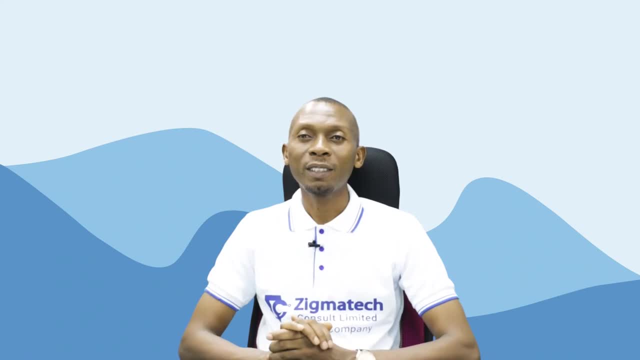 the types of crops to grow. Thank you for participating in today's class. You can practice more questions using the exam guide app. The app scores and gives a detailed explanation of all the questions at the end of your practice test. You can learn a particular topic of interest with different modes like study mode, mock mode.